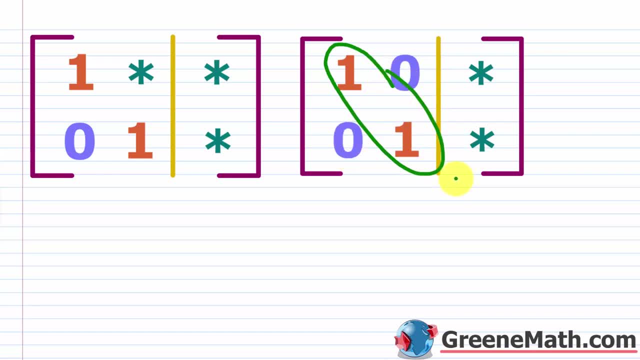 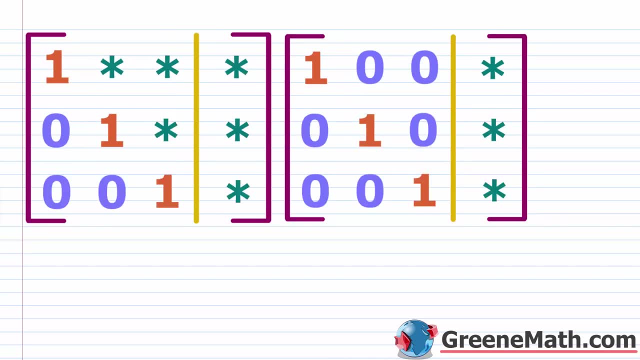 these ones going down the diagonal, a zero above and below. And so now, directly from the matrix, I can read my solution. What we're going to do today is we're just going to kind of expand on this And we're going to look at some kind of linear systems with three variables And then, in 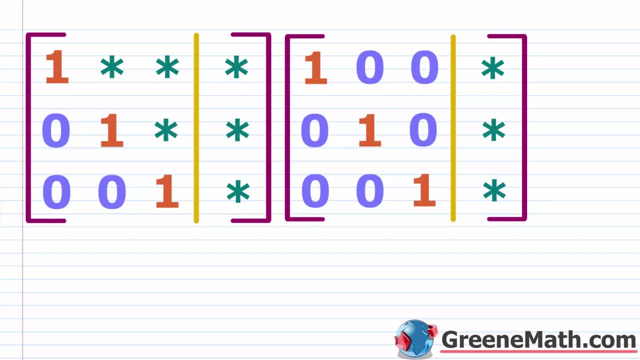 the next lesson we'll even look at some linear systems with four variables. Okay, so I want you to see the kind of row echelon form for this. So you're going to have ones down the diagonal zeros below, And of course you have to back substitute to get your answer, And then the 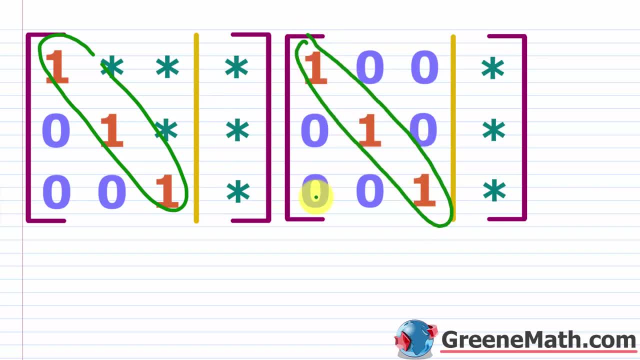 reduced row echelon form. you have ones down the diagonal, zeros below and zero above. So with the reduced row echelon form you get your answer directly from the matrix, this guy on the right. On the left, the row echelon form. 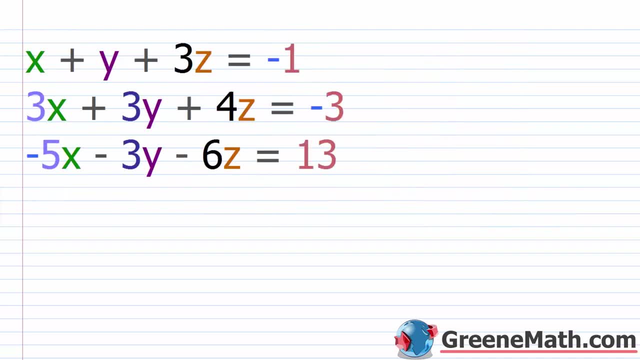 you have to do some back substituting, All right. So let's go ahead and start this with kind of an easier example. I am going to warn you that this process does get really tedious. I'm going straight off of what your textbook would show you, which is where you get a one in your column first. 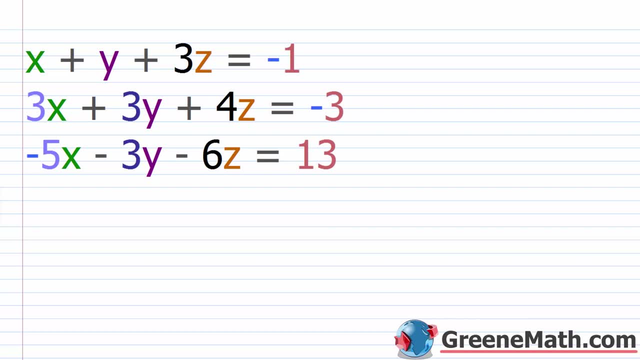 and then you find your zeros. Okay, there are faster methods to do this And you can use those if you want, But I prefer to go with just what the textbook is going to show you So you don't get confused. And then, as we kind of progress, we're going to find some easier ways to do this. 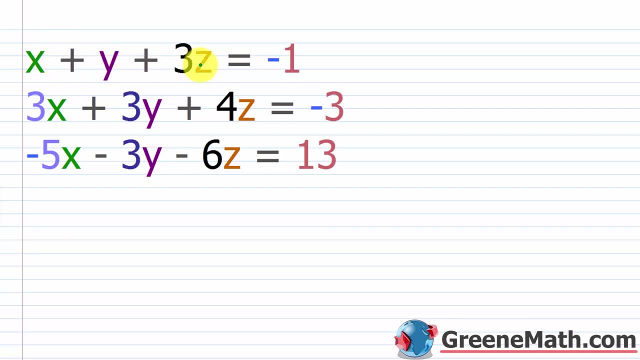 All right, so let's go ahead and read this off. We have x plus y plus three, z equals negative one. we have three x plus three, y plus four, z equals negative three. we have negative five. x minus three, y minus six, z equals 13.. So again I want all my equations in the format of: we have the ax plus by: 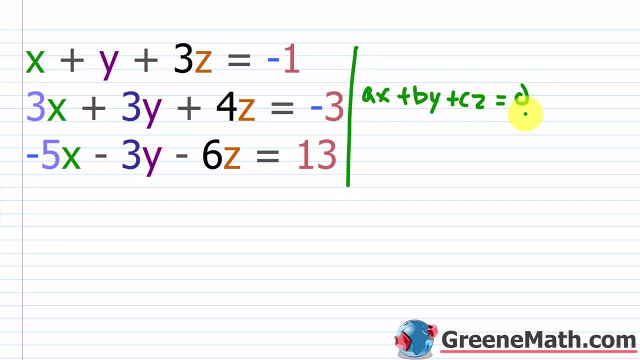 plus CZ is equal to D. Okay, the reason I want that is I want all my x terms to line up, my y terms, my z terms and my constants, Because when I write this augmented matrix, I want all the coefficients to be in the same order. So I want all the coefficients to be in the same order. So 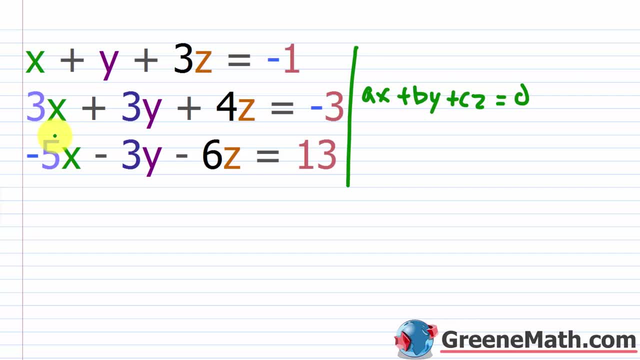 I want all the coefficients for x to be in one column, all the coefficients for y to be in one column, all the coefficients for z to be in one column, and then all the constants to be in one column. So let's go ahead and set that up, Just taking the numerical information only. we know. 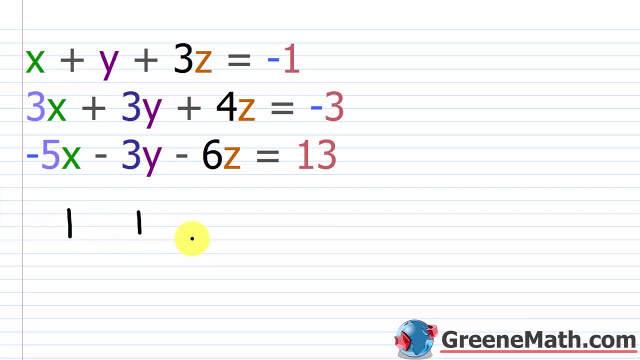 that x has an implied coefficient of one, y has an implied coefficient of one. we have a three and we have a negative one. Then, for this second equation, I have a three, a three, a four and a negative three. For my third equation, I have a negative five, a negative three, a negative six. 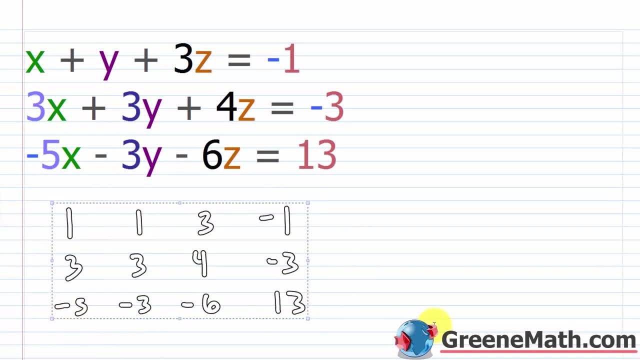 and a 13. So let's just copy that. And then I want all my equations to be in the same order, So let's copy this And let me paste that in right here We know that we want to put a vertical bar. 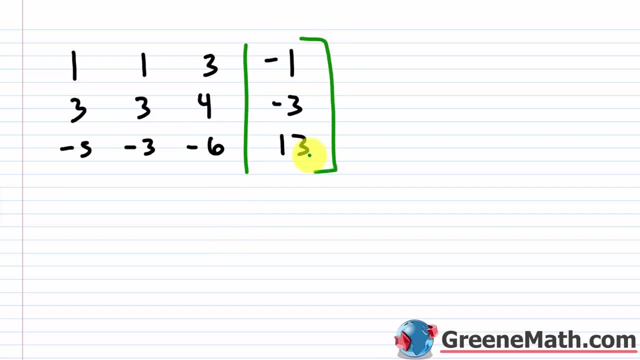 here to separate the coefficients from the constants, And then I'm going to wrap this whole thing in some brackets. So the very first thing you want to do if you're doing Gaussian elimination, you want to get ones going down the diagonal and you want zeros below. This is 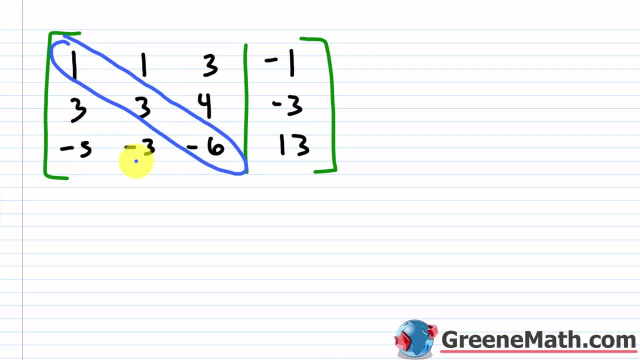 faster, right? Because you don't have to go through and keep manipulating the matrix to get it into reduced row echelon form from Gauss-Jordan elimination. I'm going to do both with you. I know it's going to be a lot of time, I know it's going to be tedious, but I want you to get a. 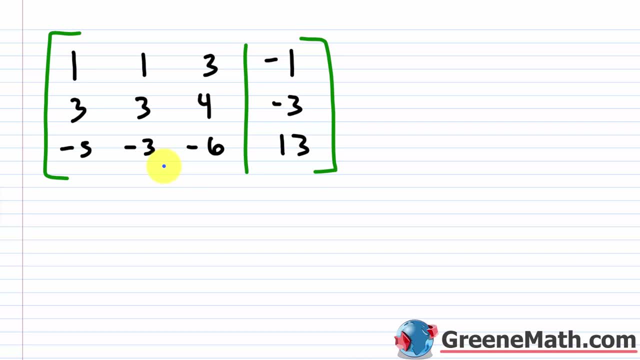 lot of practice with this. So for the first one, I'm just going to go through and do the Gaussian elimination, We're going to do row echelon form, We're going to back substitute and then I'll go back into it, okay, And we'll pound the matrix further and get it into reduced row echelon form. 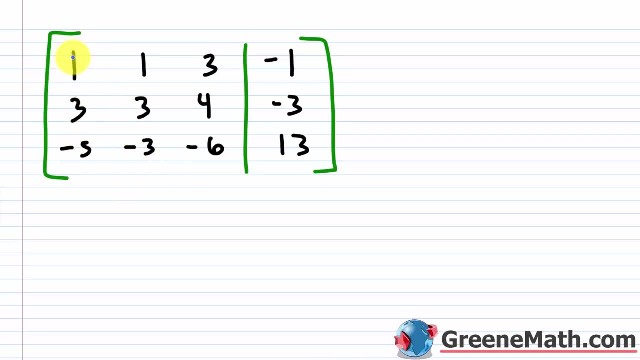 So what I want is, in the first column on the left, I want the top entry to be a one. It already is, so that's going to save us some time. So then, I want this to be a zero and this to be a zero. 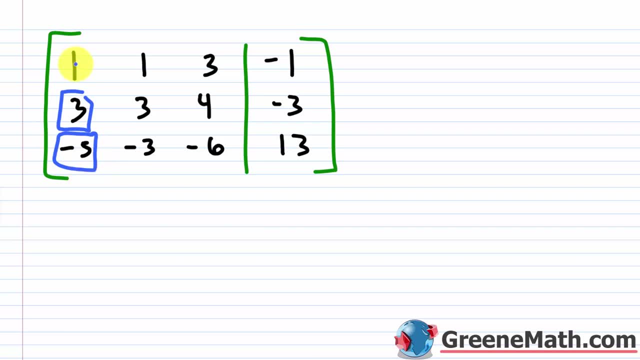 okay. So the reason your textbook always wants you to get a one in your column is because it's easy to use it to get a zero. It's always easy to get a one, hard to get a zero. So how do I get a zero? Remember, I can multiply any row by a non-zero. 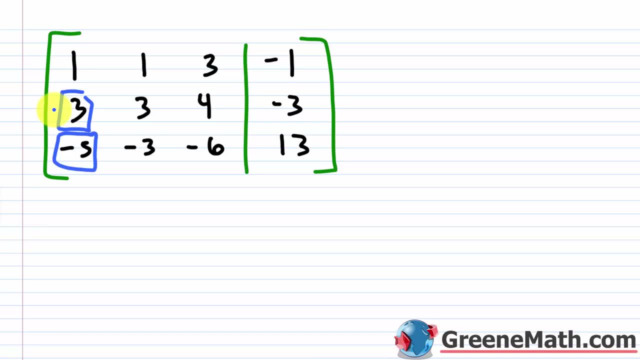 number okay and add the result to another row. So what's going to happen is I got to think about what I can add to three to get a result of zero. Well, three plus its additive inverse of negative three would be zero. And it's convenient to have a one there, because one times anything is itself. 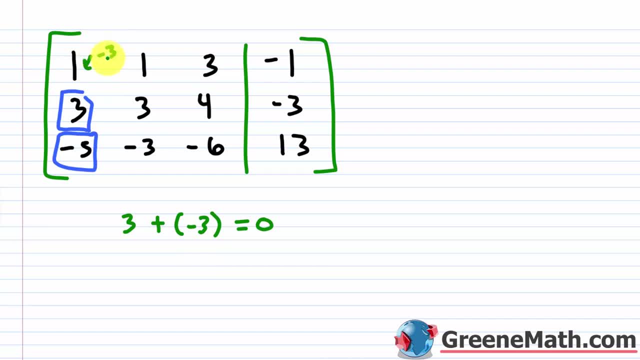 So if I multiply this by negative three, I get negative three, And then if I add negative three to three, this is going to be zero. I don't care about any of this stuff over here, I'm only worried about getting a zero here. So the way we're going to do this is we're going to say: okay. 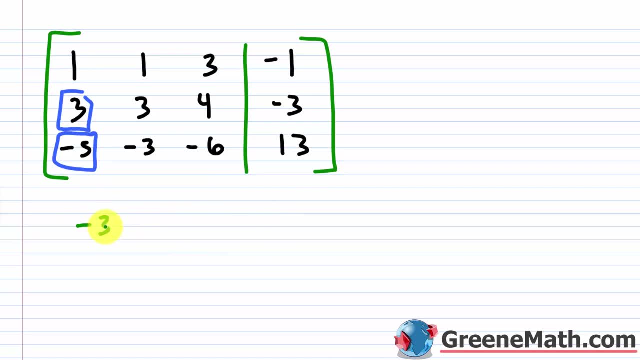 I'm going to multiply the additive inverse of three, which is negative, three times this top row or row one. And let me just label these real quick. So this is row one, row two and row three. So negative three is going to be multiplied by row one, And then I'm going to add to row. 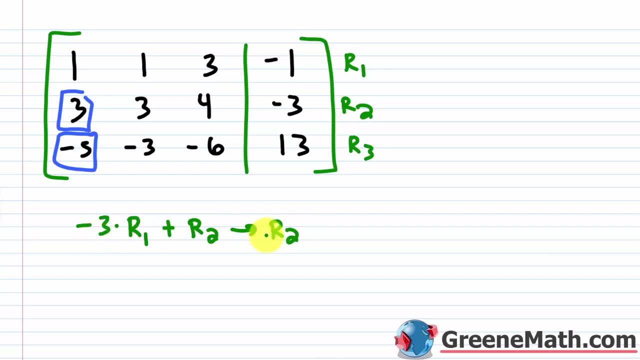 row two, and that's what I'm going to replace row two with. Okay, so that's what that notation means. And then let me do this one, too, real quick. while we're kind of working on this, we can do two at once. So we have this negative five here. So what would I need to add to negative? 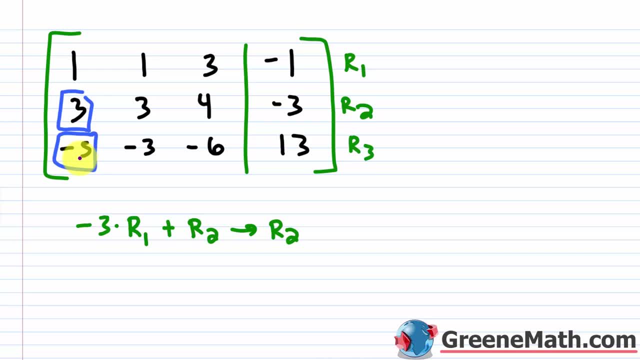 five. to get a zero, I would need to add positive five, So I would multiply this top row here by positive five, And it's really the same thing. I'm just changing this from row two to row three, And that's what I'm going to replace row three with. Okay, so let's go through this. 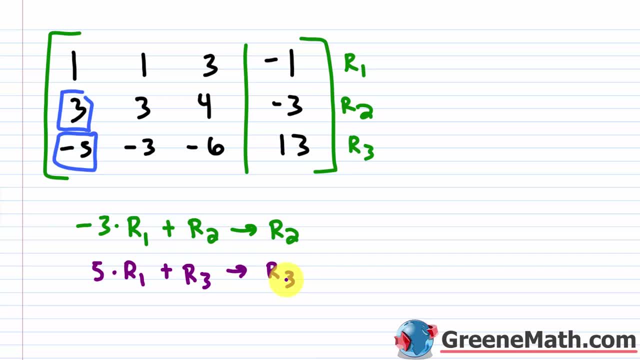 it's a good idea to kind of write these things down on some scratch paper, because one mistake here and it's going to kill you, right, you're gonna get the wrong answer. you got to start the whole thing over. So negative three times row one. that's what we're going to do. 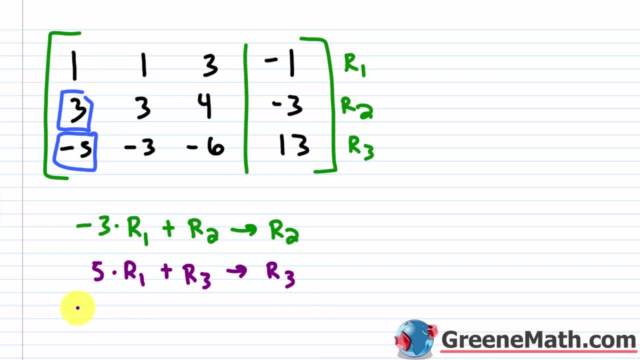 first. So I'm just going to write these answers kind of down here. So negative three times one is negative three. negative three times one is negative three. again, negative three times three is negative nine. and then negative three times negative one is positive three. So now what I'm. 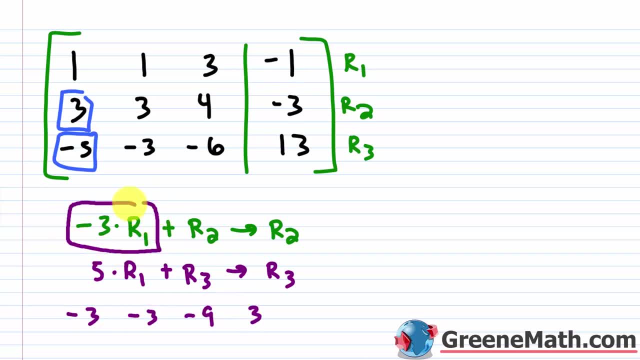 going to do is I'm going to add these kind of results. It's just this part right here. I'm now adding it to row two. okay, the corresponding entries: Alright. so negative three plus three is going to give me zero. And then I'll have negative three plus three again. that's going to be zero. 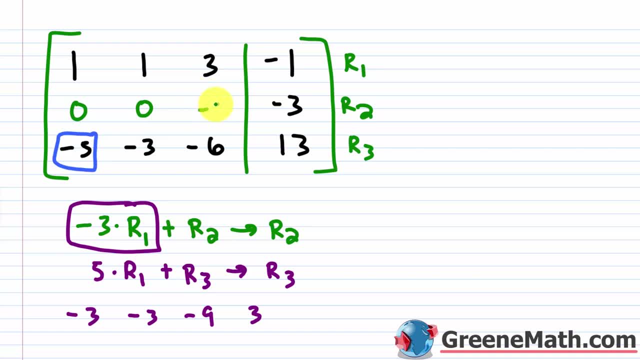 I'm gonna have negative nine plus four, that's going to be negative five. And then I'm going to have three plus negative three, which is going to be zero. Okay, so I'm done with this And I'm done with this. So I'm just going to erase this And now I'm going to move on to this one. So if I 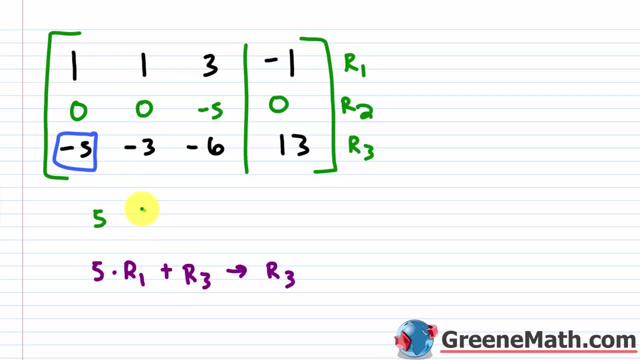 do five times one, that's five. five times one, again, that's five. five times three is 15.. And negative one is negative five. So now I'm adding these results- okay, this part right here- to row three. Okay, if you ever get lost in what you're doing, just look at your notation, it's going to. 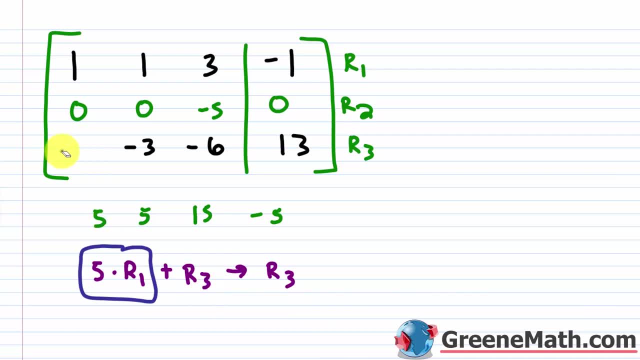 help you keep track of what's going on. So five plus negative five is zero, And then five plus negative three is going to be two, And then 15 plus negative six is going to be nine, And then negative five plus 13 is going to be positive eight. Okay, so this part's done. Now I've got. 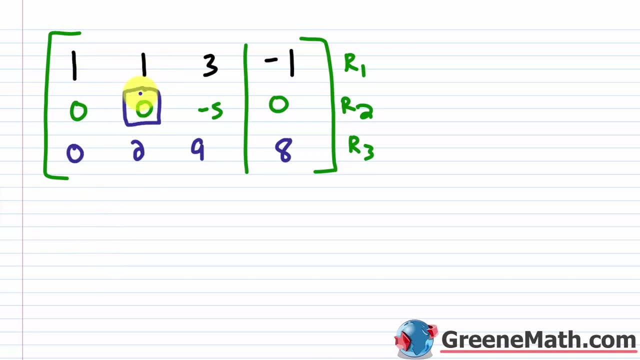 So, as I move to my next column, I want this to be a one Again. if I'm doing Gaussian elimination, okay, Gaussian elimination, I want ones down the diagonal and zeros below. I don't care about anything else. In this particular case I can't just multiply by the reciprocal. Okay, because 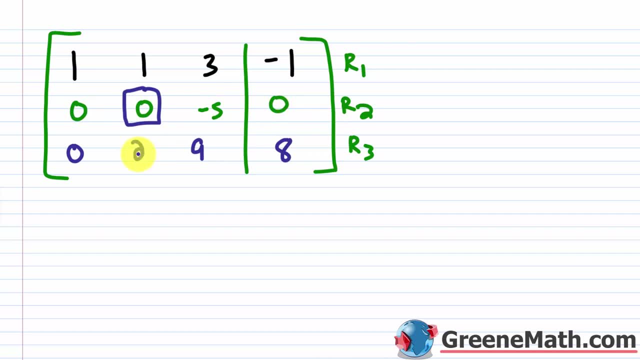 that's what I normally do, right? If I had a two in that position, I could multiply that whole row by a half, And a half times two would give me one. But because I have zero and it's unique, because zero times anything is zero, what I'm going to do is I'm actually going to switch. 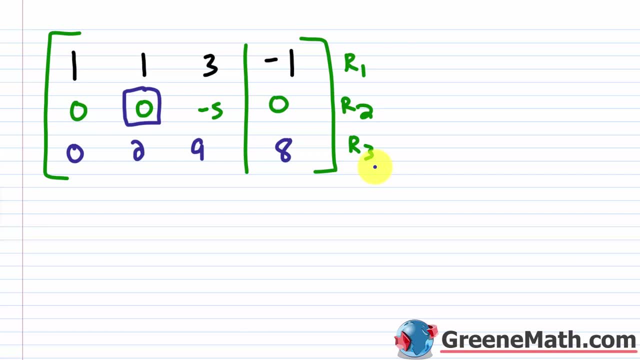 rows two and row three. Remember, we can always interchange two rows. So I'm going to say row two is going to switch with row three, And so this is going to change and be- let me kind of write this up here So we keep track- So I'm gonna have 00 negative five and zero, So I'm just gonna erase. 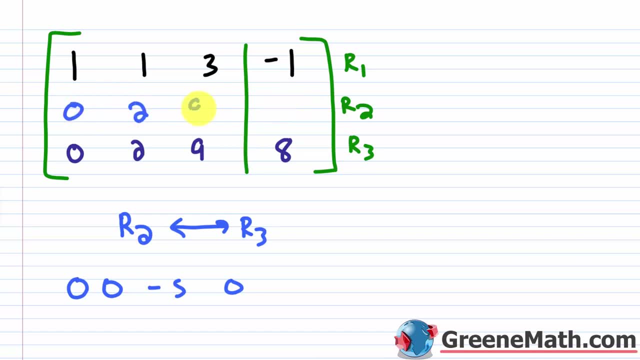 this And I'm going to copy this: So zero, two, nine and eight, And then I'll write this in here, what I just did, So 00, negative five and zero, And it's just a good idea to use a lot of scratch. 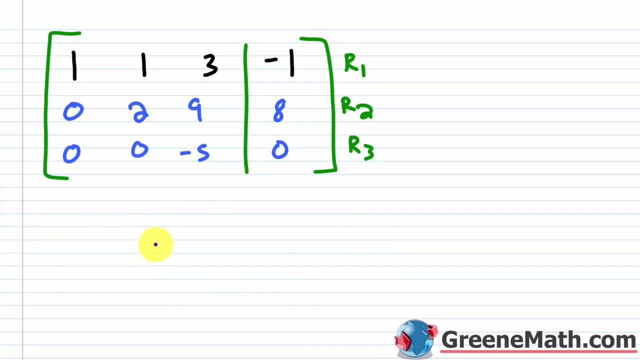 paper, because again, one silly mistake and the whole thing is blown Alright. so let's go through now and make this into a one. I'm going to multiply the reciprocal of two, okay, which is one half times that entire row, So times row two. that's going to give me my new row two, And I want you. 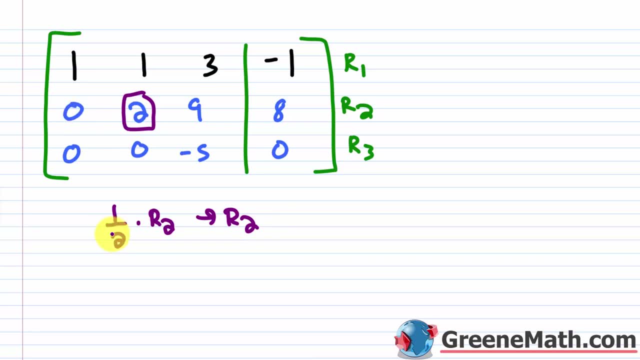 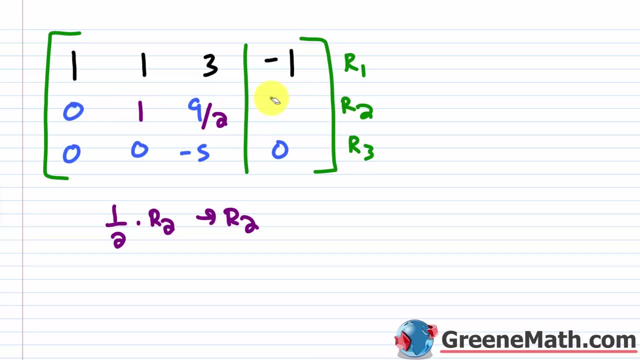 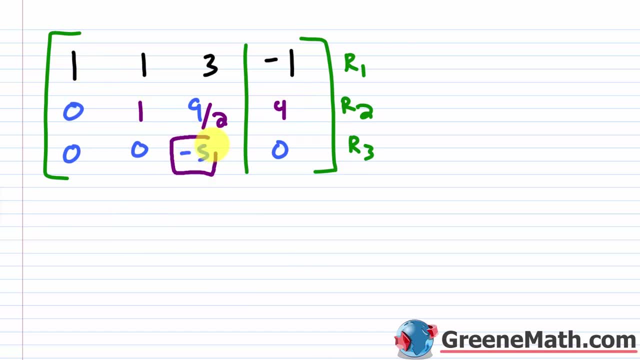 so now to complete this row echelon form, I just need a one here and I'm done. right, I can go back and substitute and find my answer. So I would want to multiply row three by the reciprocal of negative five, which is negative one fifth, because negative one fifth times negative. 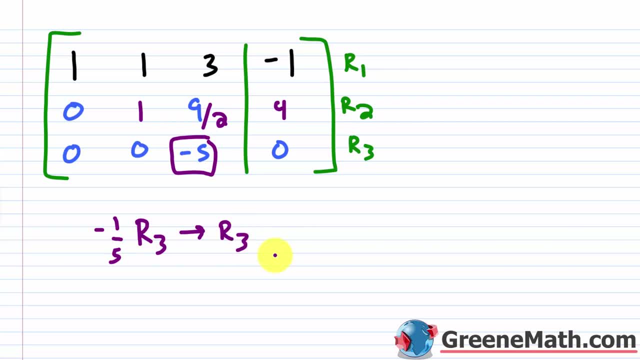 five would give me one. So that's what I'm going to replace row three with, of course, zero times. anything is zero, zero times, anything is zero, zero times, anything is zero. So I only need to change this into a one. 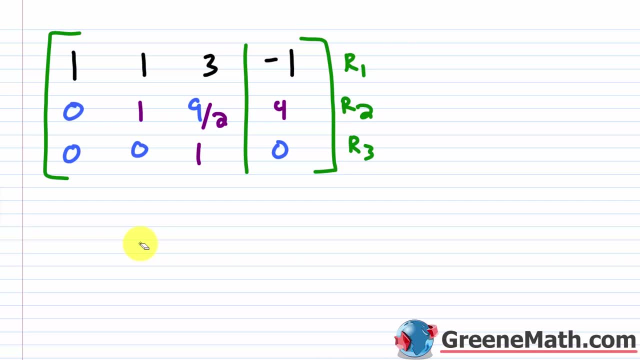 And at this point we've achieved our row echelon form. So we can just go back, substitute, figure out our answer right? So we can say that, since this column here represents the coefficients for z, we would have z or one z is equal to zero. 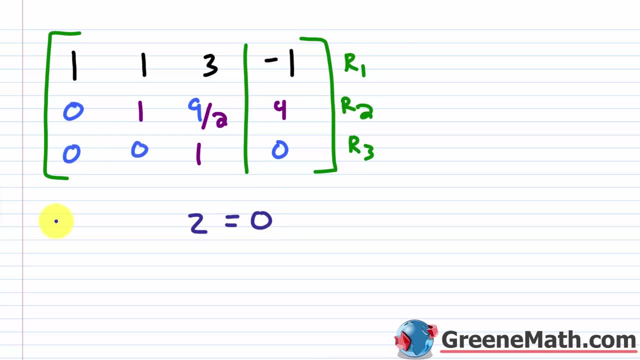 These two guys are zero, So those variables are eliminated. You can think about this as saying you have zero x plus zero y plus one z equals zero. well, zero times anything is zero. So this is zero plus zero plus one z, which is just one z, or z equals zero. 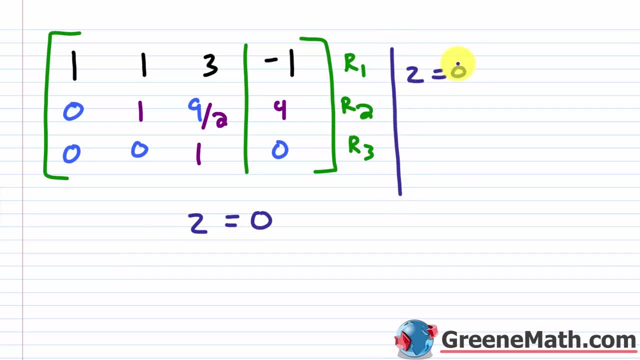 So now I can say I'm going to go ahead and do that, So I'm going to go ahead and do that, So I'm going to start back substituting. If I know z equals zero, I can take these coefficients. here I can just say: this is zero: x plus one, y plus nine halves times z. z is zero and this: 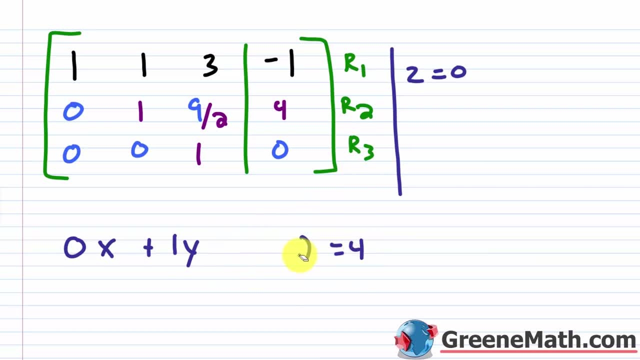 equals four. Well, I know that this is gone right. zero times anything is zero. I basically just have this gone and y is just equal to four. y is just equal to four, So that's pretty easy. And then, in terms of x, I know that one x plus one y, okay, y is four, so just four. 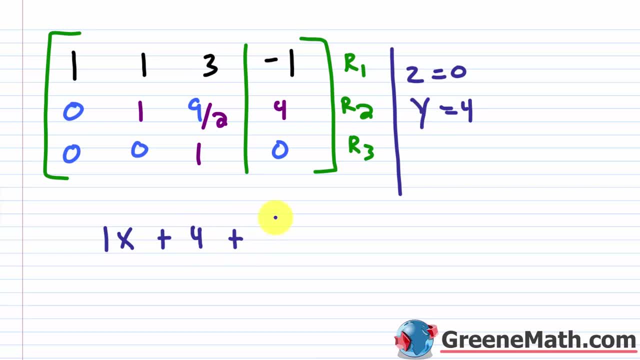 plus three, z. okay, z is zero, So I can just say: leave that off. This would be equal to negative one. Well, okay, I can just subtract four away from each side of the equation and find that x is equal to negative five. So x is going to be negative five, y is going to be four and z is. 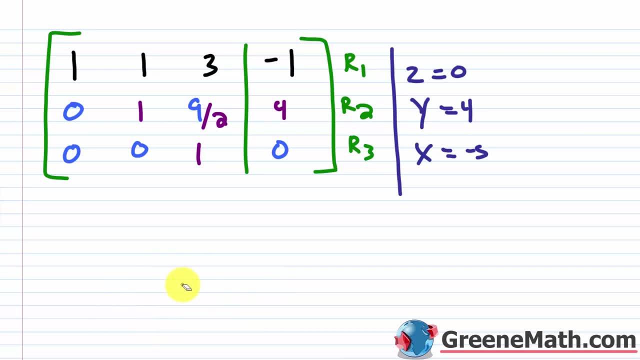 zero. So at this point, if you're just told to find the answer and you want to use a matrix method, you can just do it this way, because this is a little bit quicker than going all the way through the process with the Gauss-Jordan. okay, If you want to go through the remainder. 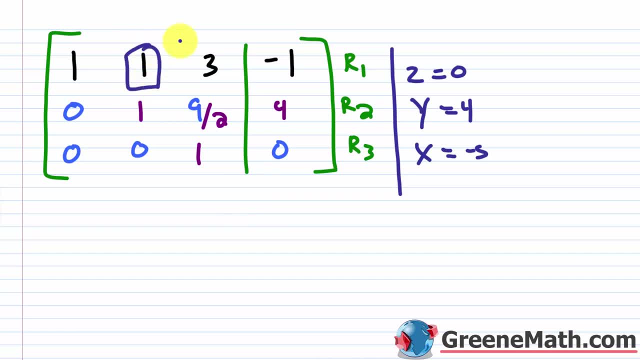 which we're going to do. what you need to do is: you need to get a zero here, you need to get a zero here and you need to get a zero here. And what that does is it allows us to kind of read the. 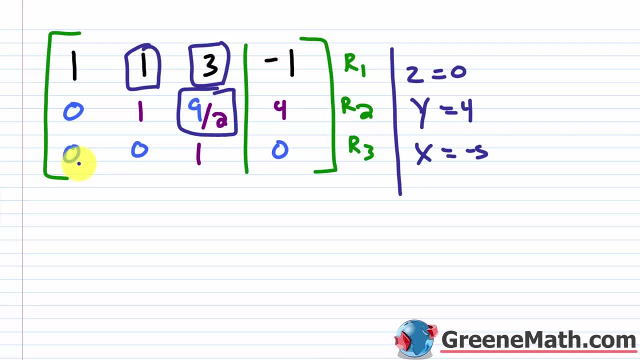 answer directly from the matrix. All right, so let's go ahead and crank this out. I'm going to start off with this guy right here in my middle column, So again, I'm going to use this one to my advantage. I'm going to multiply row two. I'm going to multiply row two by negative one. 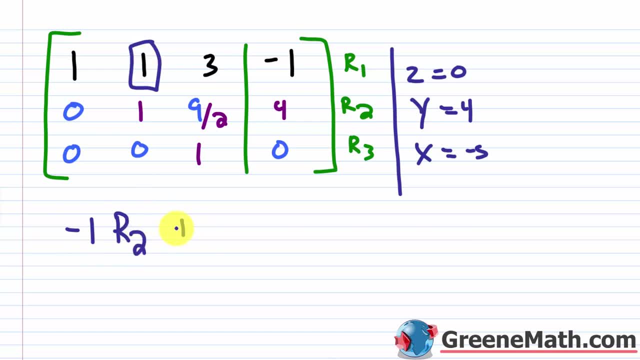 which is the additive inverse of positive one. I'm going to add the result to row two. Okay, that's how I'm going to get my new row one. So let's just go through and multiply negative one times everything in row two. So negative one times zero is zero. We have negative one times one. 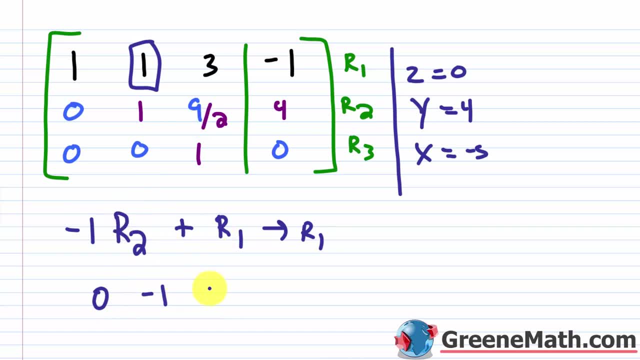 which is negative one. We have negative one times nine halves, which is negative nine halves, And then we have negative one times four, which is negative four. So what I'm going to do now is I'm going to add these results here, this part right here, to the corresponding entries in row one. 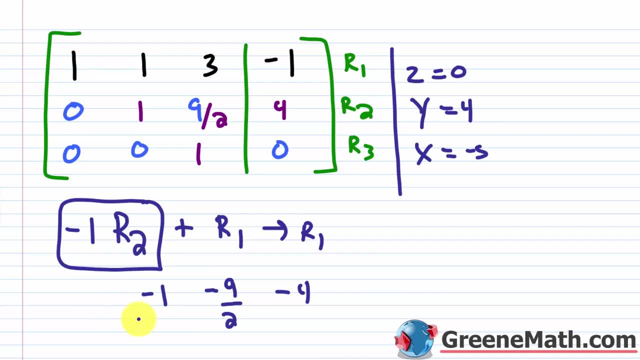 So we know zero plus anything is going to leave it unchanged, so I don't need to worry about that. Negative one plus one is going to be zero. I know that negative nine halves plus three. Let's do that off to the side in a minute And then I would have negative four plus negative one, which is negative. 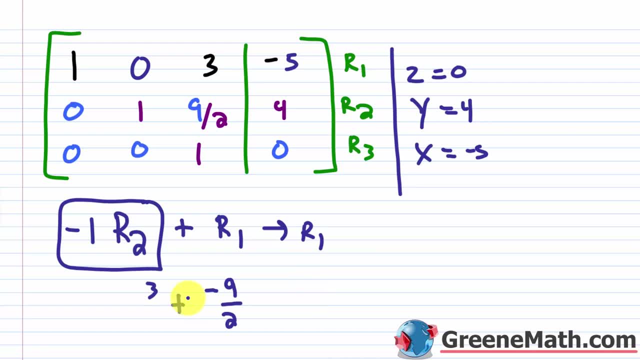 five, Okay. so let's work on this one. right here We're trying to figure out what this is going to be. So, to get a common denominator, I'd multiply this by two over two, Okay, and I would have six. 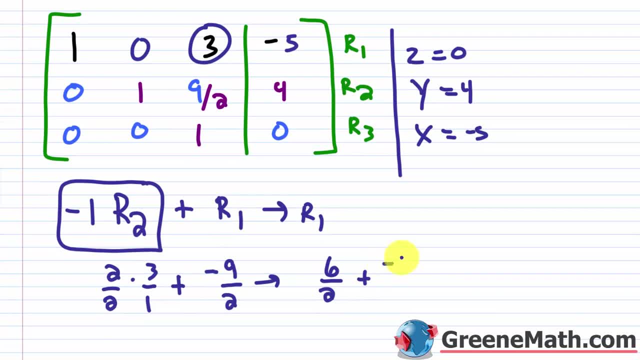 Let's just write this as six over two plus negative nine over two. I know that negative nine plus positive six is going to be negative three, So this would end up being negative three over two. So this is done. So let's erase this. 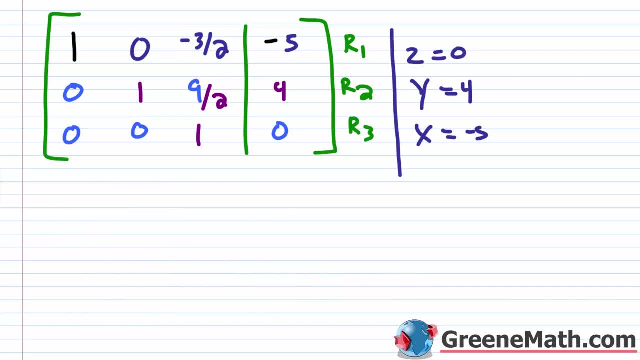 So now what I need is a zero here and here. to finish this up. It's actually going to work out pretty conveniently here, because we have a zero here, a zero here and a zero here. So what does that actually mean? Well, remember, if I'm trying to work on things in column three, 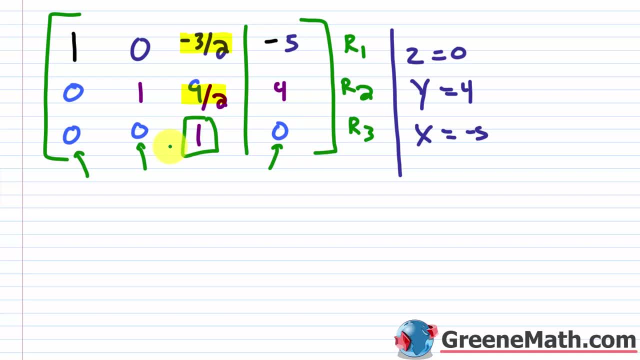 I'm going to use this one in row three to kind of work off of, And what makes it easy is that when I multiply this by two, I'm going to get a zero here. So I'm going to get a zero here. If I multiply by zero, I get zero. If I add zero to something, it leaves it unchanged. 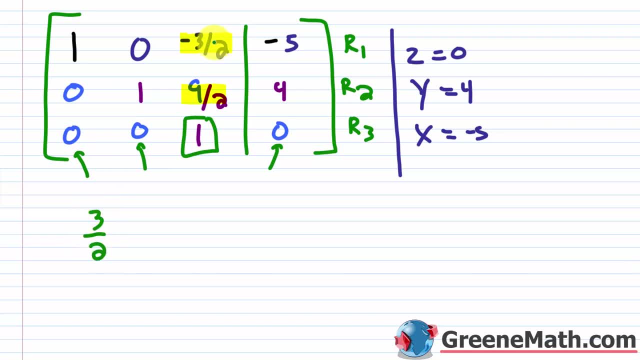 So what happens is, if I want to multiply three halves the additive inverse of negative three halves times my row three, in every case it's going to be zero, zero and zero over here. So when I add those to the corresponding entries, nothing's going to change. 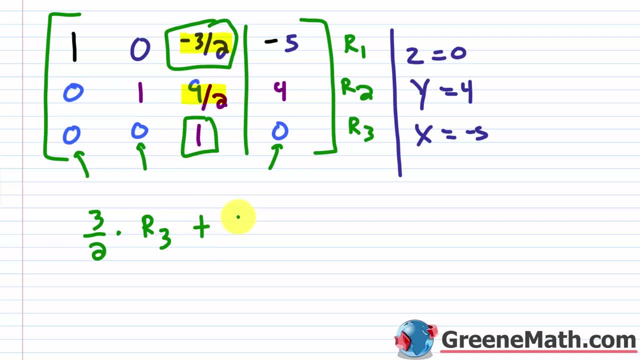 So the only thing that's going to change is this: Okay, so if I add this to row one and I replace row one with this, I only need to change this, and I'm just going to change it into a zero. It's the same thing here. So if I multiply negative, okay, negative nine halves times row. 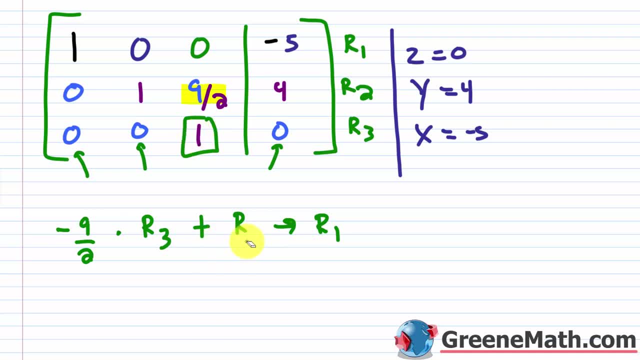 three, okay, for that one, and then I add the result to row two. that's what I'm going to replace row two with. Once again, these zeros do not affect this. okay, because negative nine halves times zero is going to be zero. Adding zero to something does not change it, So I'm only going 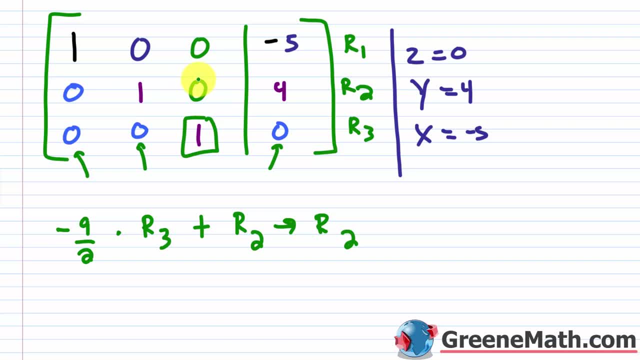 to change this guy right here and it's going to be a zero. All right. So we can see that we got the same answer by putting our kind of augmented matrix into a zero. So if I add this to row two in this reduced row echelon form, we have our ones. going down the diagonal, We have zeros above. 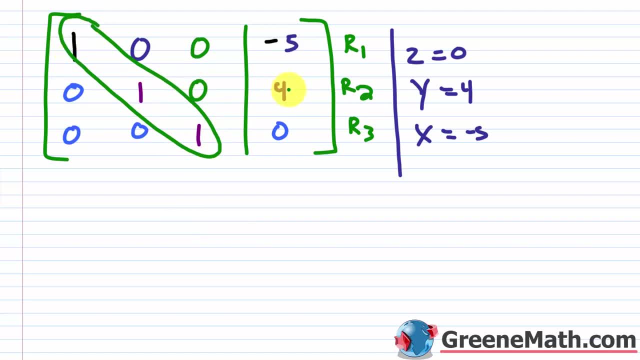 and below. So we find that X is negative five, We find that Y is four and we find that Z is equal to zero. All right, So let's go ahead and take a look at another one Again, as we work more and 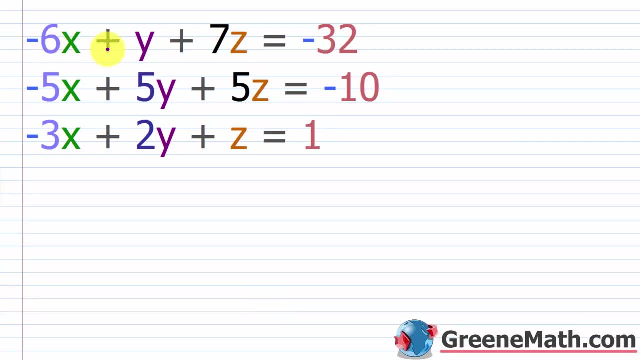 more of these. they get easier and easier. So we have negative six. X plus Y plus seven Z equals negative 32.. Let me just write the negative six, the one for the coefficient for Y, that's implied the seven, and then the negative 32.. 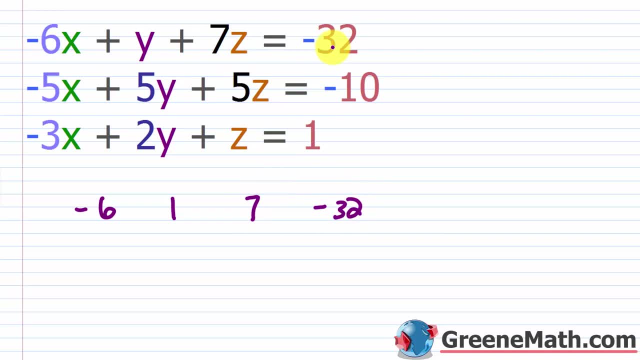 Okay, Just taking the information from the first equation, Then from the second one, you have negative five. X plus five Y plus five Z equals negative 10.. Again, when you see something that can be simplified, meaning everything here is divisible by five, go ahead and take the. 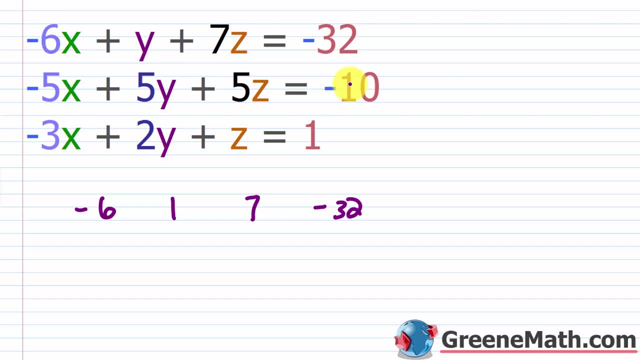 opportunity to do that, because it's going to mean that you're working with smaller numbers. So if I divide everything by five, this would be a negative one, This would be a one, This would be a one and this would be a negative two, So you'd have negative one, one, one and negative. 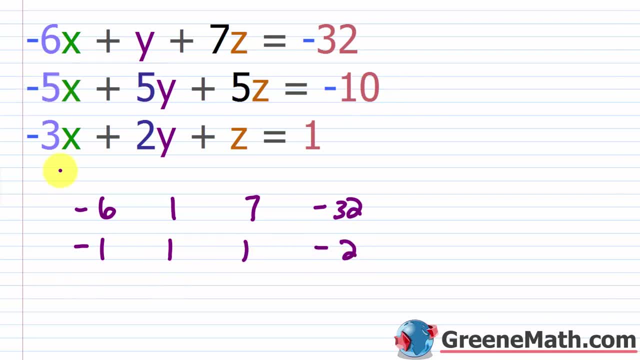 two, Okay, And I can erase that. And then, for the last one, we have a negative three, We have a two, We have a one- Again, that's implied to be a one, And then we have a one, Okay. So let me put my 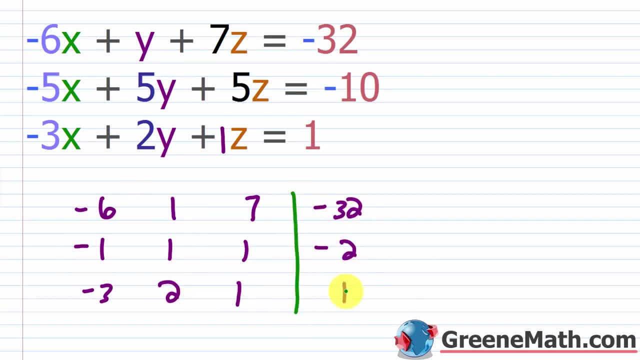 vertical bar here to separate the coefficients from the constants. And once again I just want to stress this: This is already written in the format of AX plus BY, plus CZ equals D. If it's not already written in that format, you've got to do that first. Okay, All right, So let's set this: 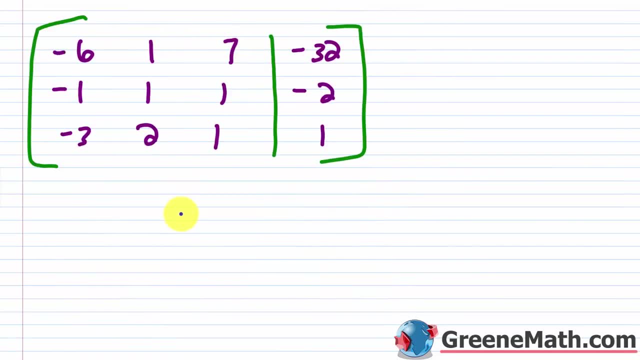 up and let's copy this, All right. So let's paste that in. So again, I want this top left entry to be a one. So the easiest way to do that is just to multiply this first row here by the reciprocal of this number. So again I can label this as row one, row two. 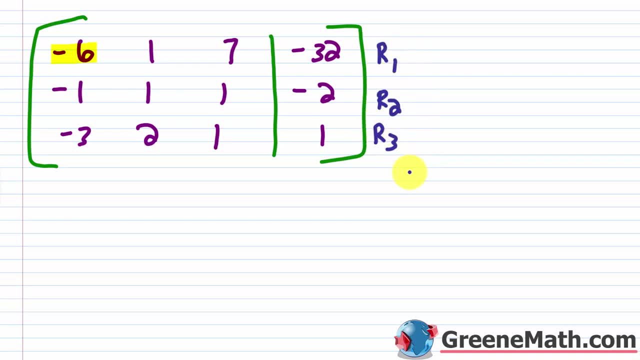 and row three. You don't have to do this, but it's just nice to kind of show what's going on. So I'm going to multiply negative one sixth, which is the reciprocal of negative six, by row one. That's going to give me my new row, Okay. So if I do that, negative one sixth. 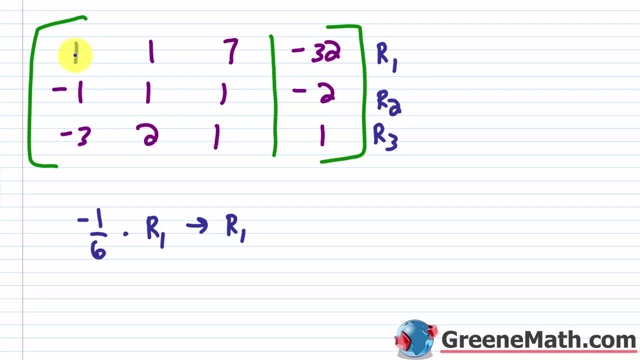 times negative. six is going to be positive one. Negative one sixth times one is going to be negative one sixth, Then negative one sixth times seven is negative seven sixth And then negative one sixth times negative 32.. Let's do that off to the side, So we would have 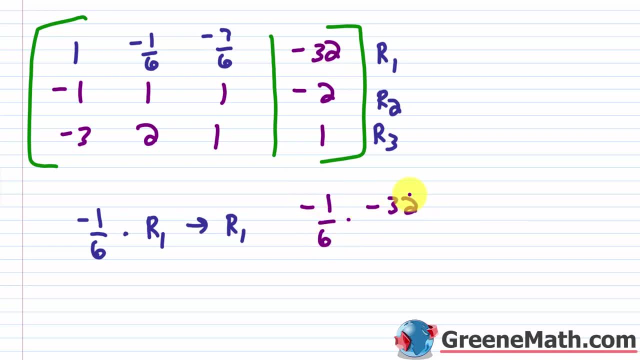 negative one sixth times negative, 32.. We know that negative times negative is positive, So we can get rid of that sign there. So we'll just erase these. We don't have to do that. And then 32 and six. they're each divisible by two right. So 32 divided by two is 16.. 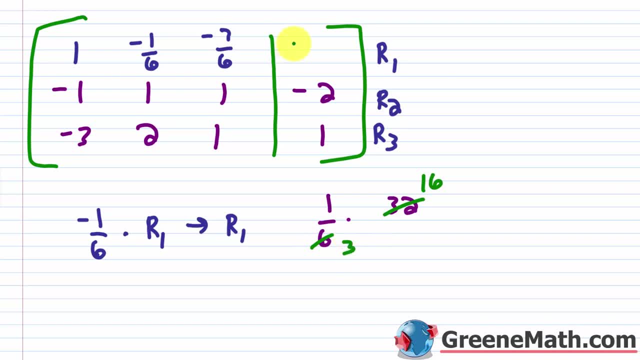 Six divided by two is three, So this is going to be 16 thirds. All right, So the next thing I want to do is I want to get zeros below this one. So I want this to be a zero and I want this to be a. 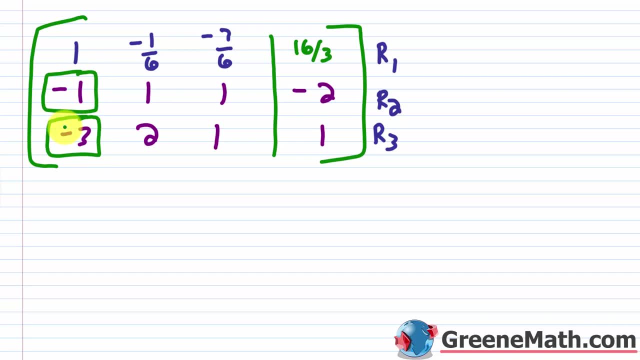 zero. So what can I do? Again, I just think about the fact that I have a one here already. Okay, I have a one there, And the reason you get the one first is so that you can work with that. So all I need to think about is 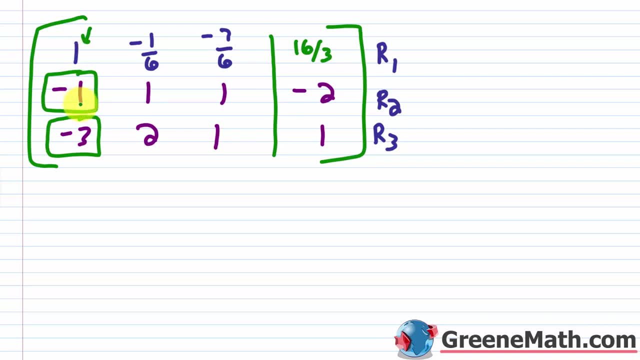 the additive inverse of negative one which is positive one. Okay, So I would just multiply row one by one, or you can just think of it as I'm just going to add row one to row two. Okay, So what I'm going to say is: I'm going to multiply row one by one. I'm going to add the result to row. 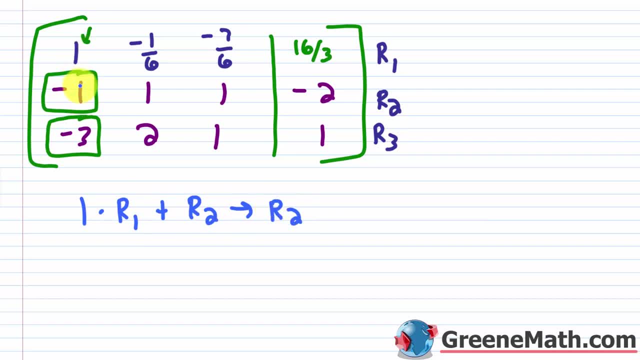 two. That's going to give me my new row two. Okay, So all I'm going to do is just add. So one plus negative one is zero Negative one. sixth plus one is one. I'm going to write this as six over six. 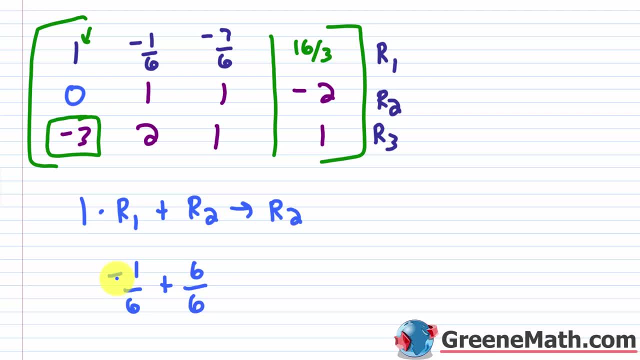 And six minus one would be five. So this would be five, six. Then for this one you'd have negative seven, six plus one. I'm going to write a six over six. negative seven plus six is going to be negative one. So this would be negative one. sixth: 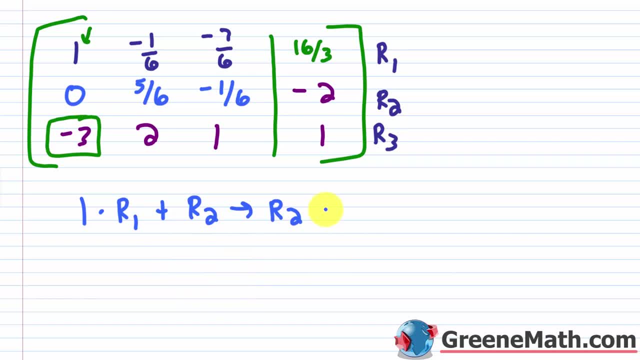 And then, lastly, you would have 16 thirds plus negative two. So 16 thirds plus you'd have negative. I'll go ahead and do that, I'll go ahead and do that. And then, lastly, you would have negative. I'll go ahead and say: this is six over three. So 16 minus six is 10.. So we can say this: 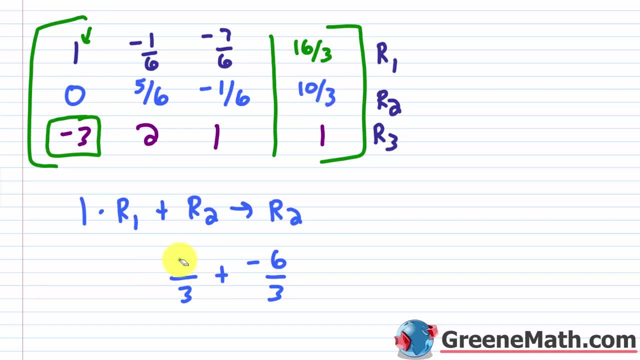 is 10 thirds. Okay, So that's taken care of. So to get a zero, here again, I use the same concept. I'm going to use that one there And again. the opposite of negative. three is three, So I'm going to multiply row one by three. add the result to row three, So I'm going to multiply row. 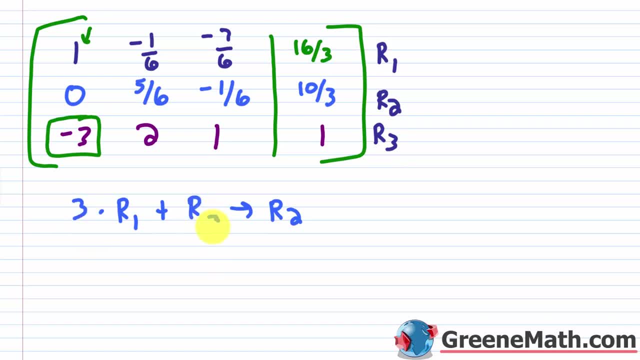 one by three. add the result to row three. That's going to give me my new row three. So one times three is three. Negative. one over six. negative one over six times three is one. This will cancel with this and give me a two. So this is negative one half, This is negative one half, And then negative seven. 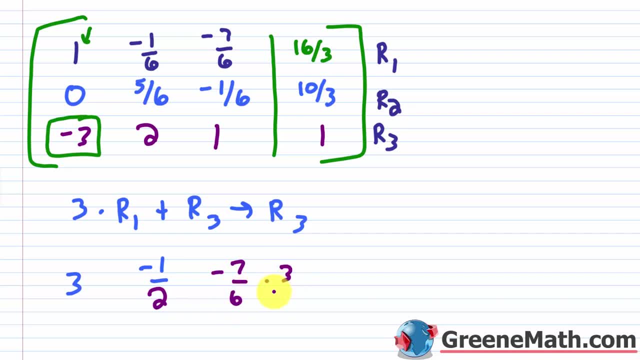 six negative seven. six times three is one. This cancels with this and gives me a two. So this is negative seven halves. And then you have 16 thirds times three. The threes are going to cancel, So this will cancel with this and I have 16.. All right, So let's add now three plus negative. 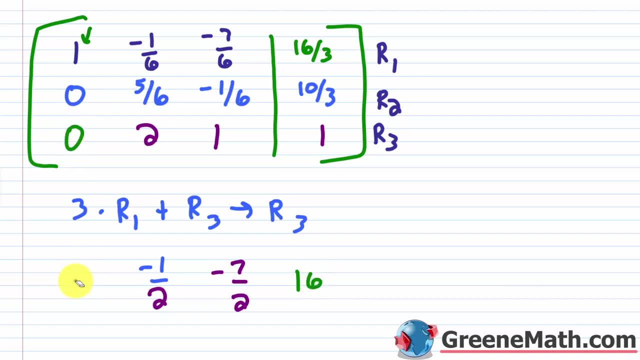 three is zero. So let me erase this. We'll have negative one half plus two, So negative one half plus two. So let me do plus four over two. So this would be what Four minus one is three, So this would be three halves, So three halves, Okay. So this is gone. Then negative seven halves plus 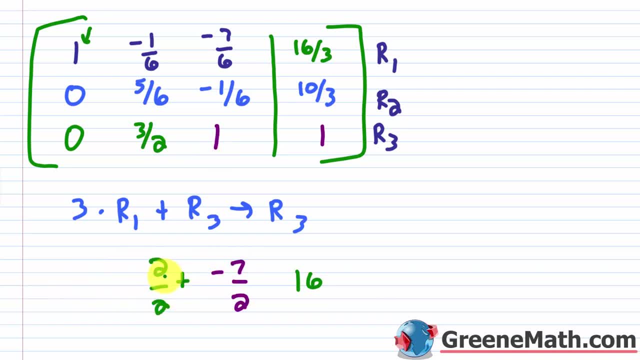 one. Let's add two over two. Negative seven plus two is negative five, So this would be negative five halves. And then, lastly, you would have 16 plus one, which is 17.. Okay, So this is 17.. All right, So now we. 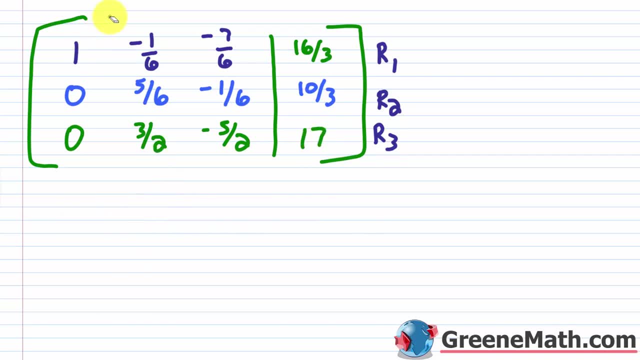 have the first column done and we're going to move into the second column. here And again, I always want to start by getting a one. I get the one, and then I can get the zero above and below pretty easily. So to get the one, I just multiply row two by the reciprocal of this five sixths, which. 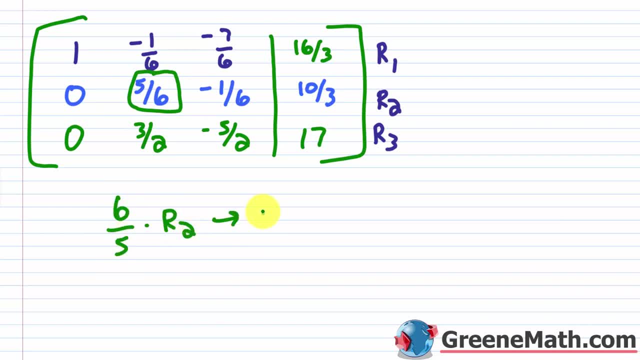 is six fifths. Okay, So six fifths times row two. That's what I'm going to replace row two with, All right, So we know that this guy to the left isn't going to be affected, because zero times anything is just zero, Okay, But this guy is. 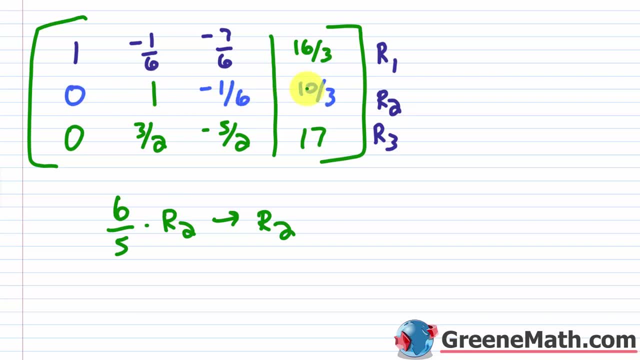 going to be a one, So I don't really need to worry about that. I really just need to do the calculations for these two. So I would have six fifths times negative one. sixth, Okay, So this would cancel with this and give me a negative one fifth. So this would be negative one fifth. 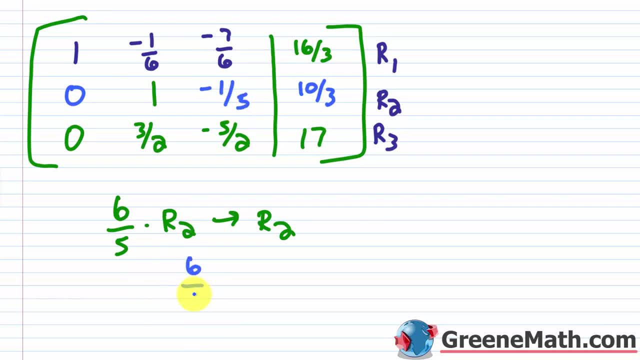 Let me erase that. And then, lastly, you would have your six fifths times 10 third's. We know that this would cancel with this and give me a two, And this would cancel with this and give me a two. Two times two is four, So this would be four. So now we want to. 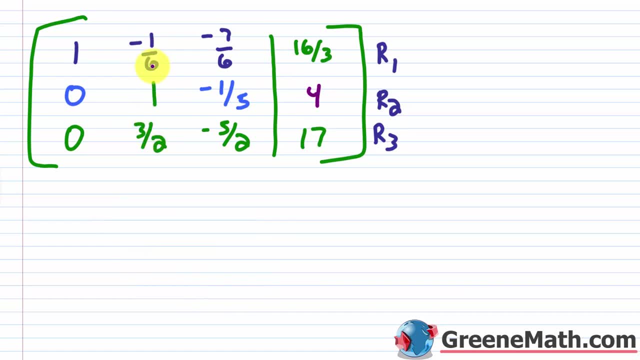 get a zero above and below this one. So again I'm thinking about the additive inverse of negative. one sixth, So that's going to be one sixth. So let me multiply row two. Let me multiply row two by one sixth. So one sixth times row two, then plus row one. This is going to be my new row one. Okay, 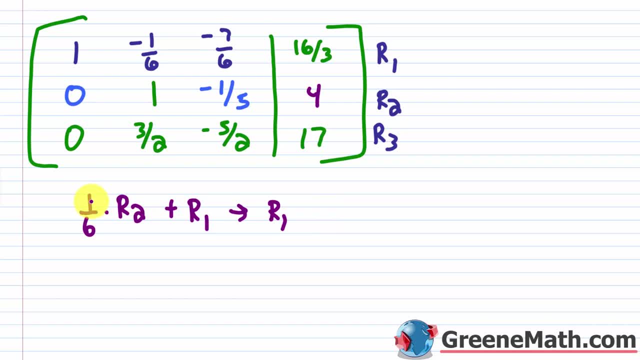 So again, to the left of this, it's not going to matter, because zero times anything is zero. zero plus anything is just itself. So I really need to just think about, I know that this would turn into a zero. So I really just need to work on this negative one fifth times, one sixth, Okay. 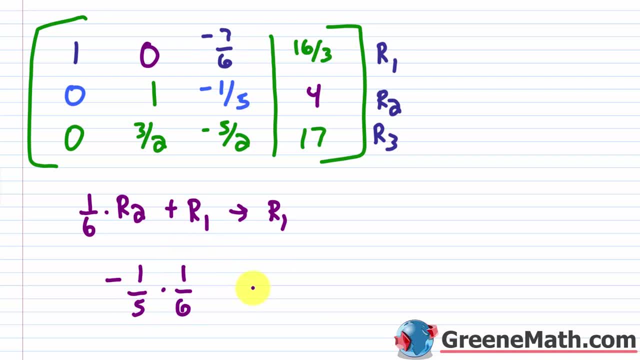 And then I'll add this result to this negative seven, sixth, So I know that this would be negative one over 30. So negative one over 30, and then plus negative seven over six. So I'll multiply this by five over five. negative seven times five is negative 35. So you would have negative. 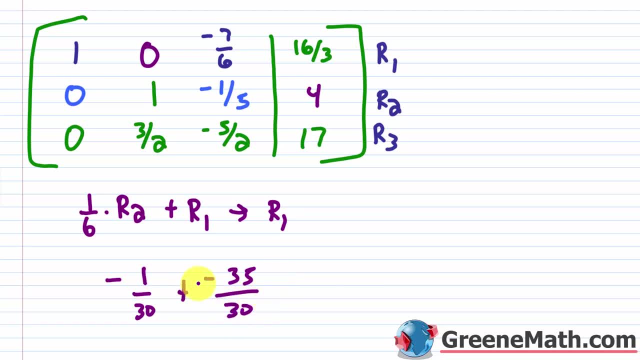 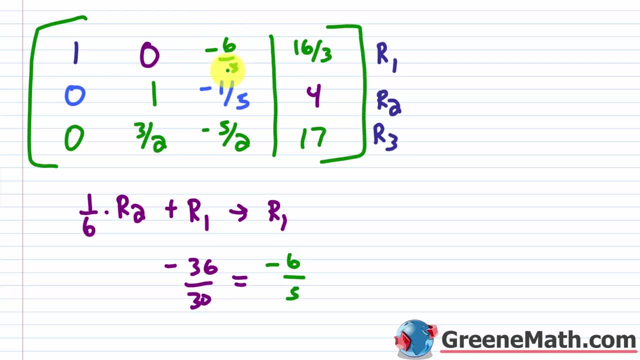 So I'll replace this with negative six fifths and one more. Okay, We need to do one more, So let me write that a little bit better Now. I also need to multiply four by one sixth, So four times one sixth. This would 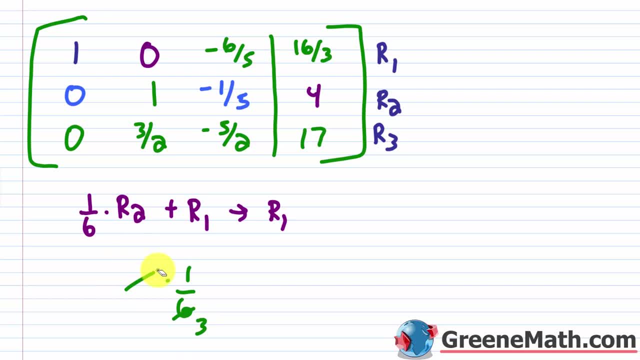 cancel with this: This would be a three, This would be a two, So this would be two thirds. Okay, So two thirds. And then add that result to 16 thirds. Okay, So 16 plus two is 18.. 18 divided. 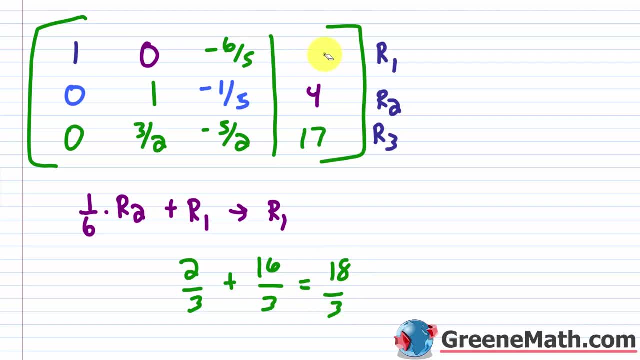 by three is going to give you six, And let's get this guy to be a zero now. So I'm going to multiply row two. I'm going to multiply row two by one. Again, I want the additive inverse of this. So 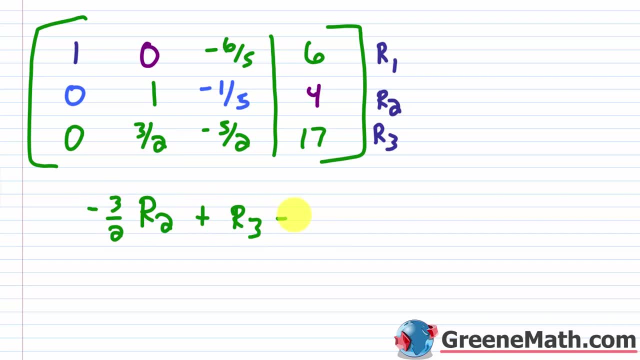 negative three halves. Then plus my row three, That's going to give me my new row three. I know that I don't need to really do anything this way, because I'll be multiplying this by a zero and that's going to be zero, And then adding it to. 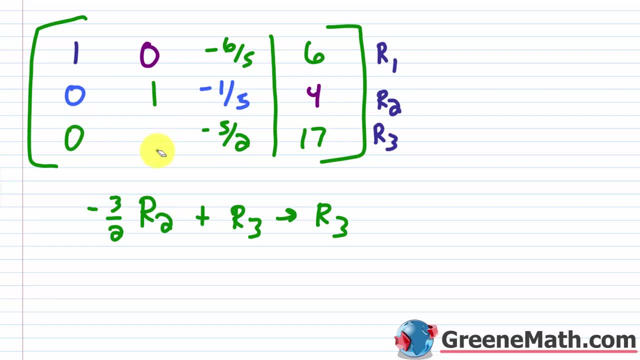 this would leave it unchanged. So really I just need to change this into a zero, because I know it would be zero And I need to work on this one and this one. So I would multiply negative three halves times negative one fifth, And that would give us three tenths, Okay. And then I would add: 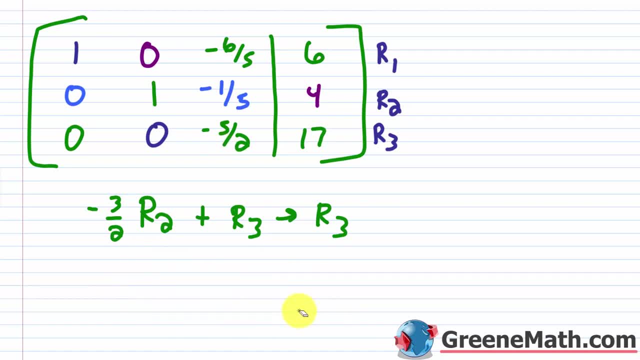 three tenths to negative five halves. So three tenths, Three tenths plus negative five halves. Multiply this by five over five, So this would be negative 25.. Negative 25 over 10.. Okay Over 10.. So negative 25 plus three is. 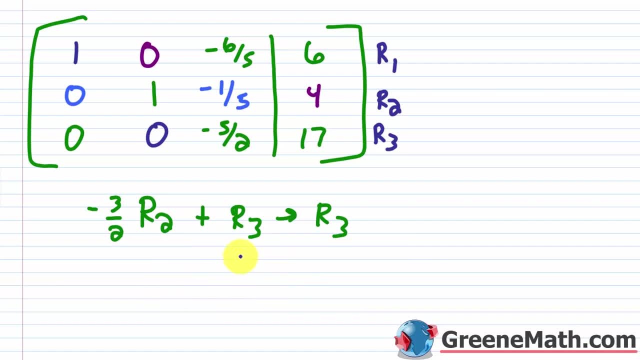 negative 22.. So you would have negative 22 over 10.. This is negative 22 over 10.. And then, lastly, I'm going to multiply negative three halves times this four. Okay, That's going to cancel. Give me two Negative three times two is negative. 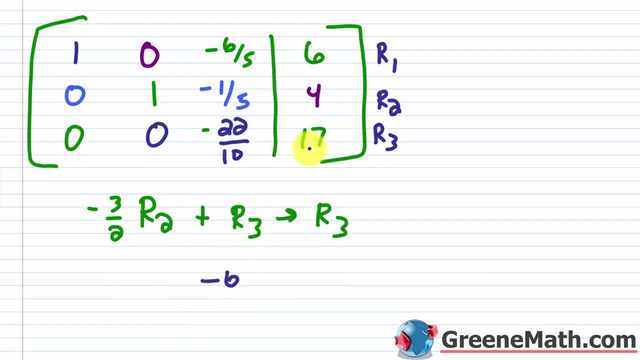 six, So negative six, And then add the result to 17.. That's going to be 11.. What we want to do now is get a one as this entry here: Okay, So how do we do that? We multiply row three. 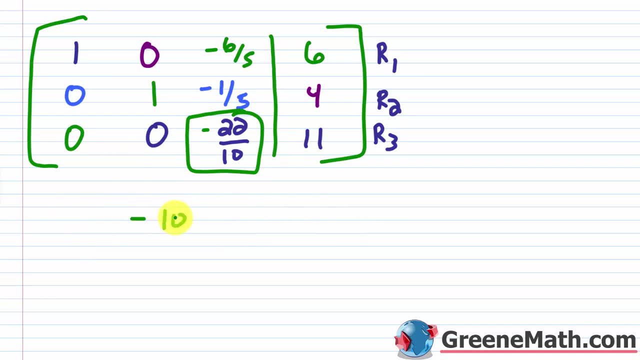 by the reciprocal of that guy. So I'd have negative 10 over 22 times row three Again, that's going to give me my new row three. So we know that this would, we know that this would be a one, And we can just eyeball this and say that I know that. 11. 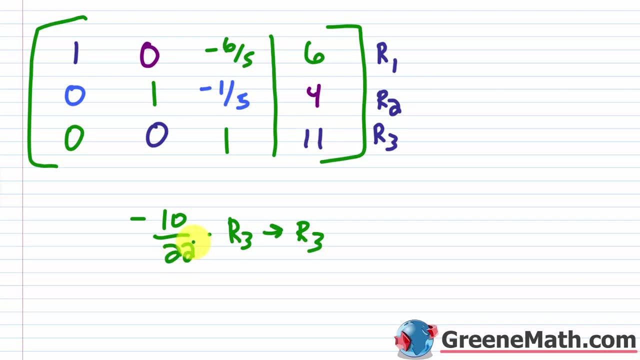 would cancel with 22,. right, 22 divided by 11 is two, So let's just erase this. This would become a two, and negative 10 over two would be negative five. Okay, So at this point you have row echelon four. You have ones down the diagonal, Okay, Let me highlight that. So one's down the 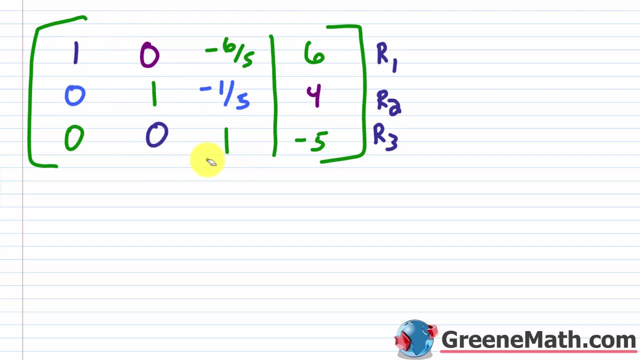 diagonal. You have zeros below. Okay, So that's row echelon form. This is what we get. So we get from Gaussian elimination, but we're going to continue with the Gauss Jordan elimination and put this in reduced row echelon form. So I want to zero here and here Again. it's not that hard. 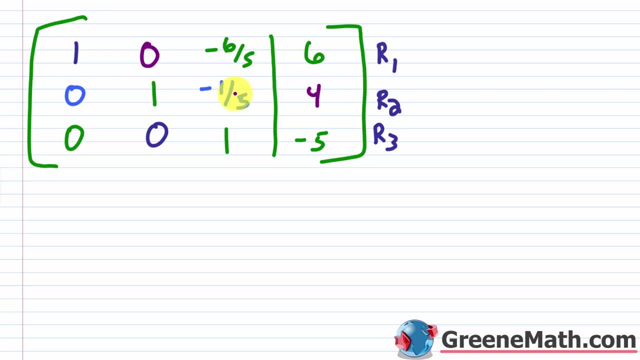 because we're, we're almost there. Okay, I know this is very tedious and that's just because we're taking our time. So for this guy right here, this negative one fifth, I can make it into a zero by multiplying row three. Okay, Row three by one fifth. add the result to row two, So one fifth. 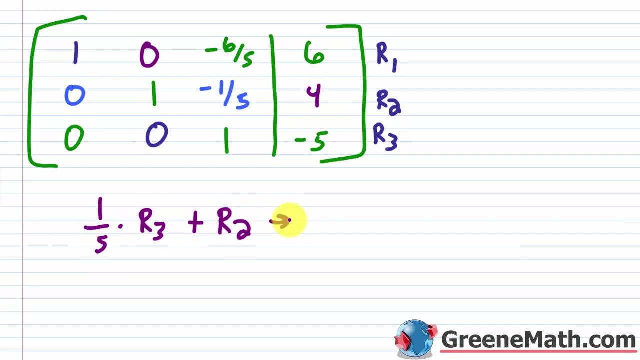 times row three plus row two, We give me my new row two. Okay, So I know I don't have to work this way. right, I don't have to worry about that, because if I'm multiplying a zero, okay, In each case here by this number, I get zero, And 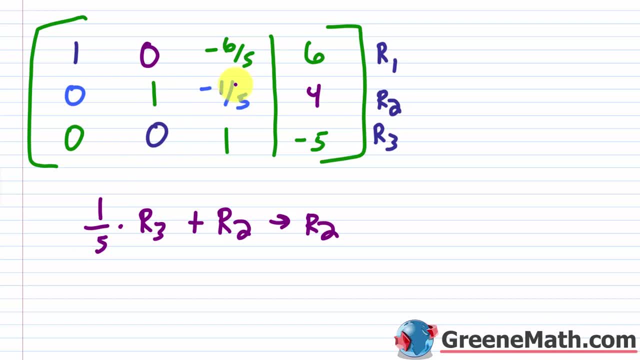 then if I add zero to something, it stays unchanged. So I really don't even need to work on this one because I know it's going to be zero. I just have to work on this one, Okay, So that makes it kind of quicker. So it's one, fifth, one, fifth times- this guy right here, which is negative. 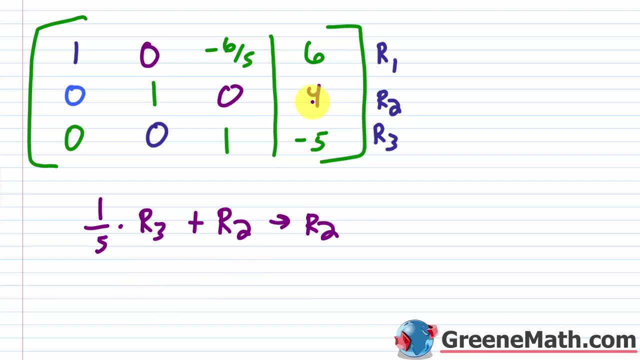 five, That becomes negative one, Okay, And that gets added to four. So I know I don't have to work on this one. So that makes it three, Okay. So now the last one. we're going to multiply row three by six fifths. Okay. So by six fifths we're going to add the result to row one, and that's going to 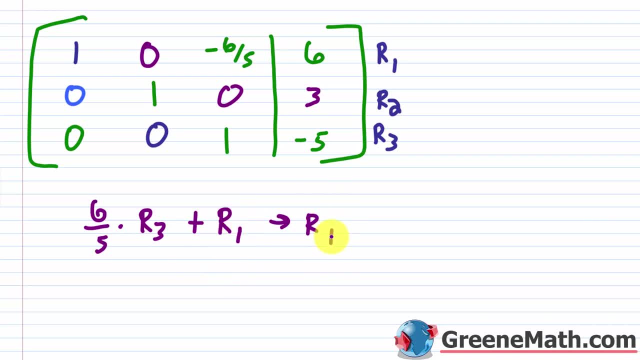 give us our new row one. Okay, Now, again, when I think about this, I don't need to do anything this way. Okay, I know, I'm going to replace this with a zero, Okay, And I just need to work on. 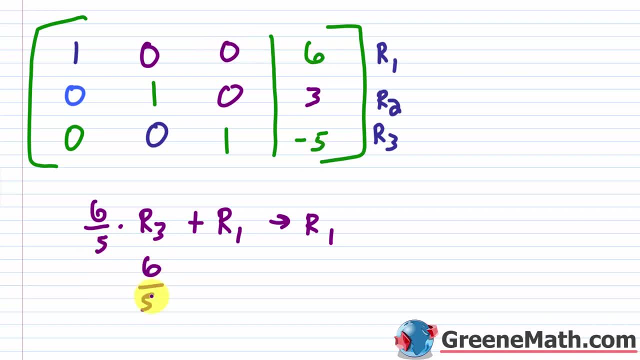 this one. So six fifths times negative five. six fifths times negative five. This would cancel. It would give me negative one. So it's negative six, So negative six plus six would give me zero. So now I have my solution, finally. Okay, So I can say that one Z equals negative five or Z equals. 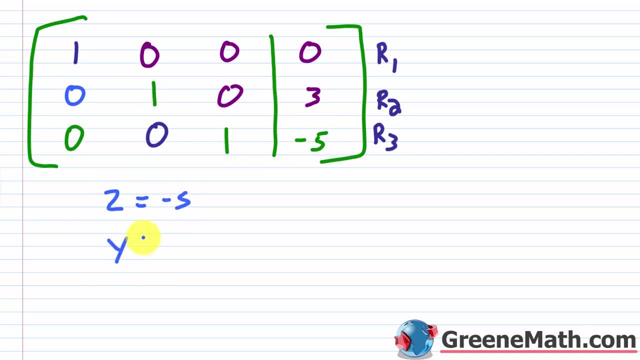 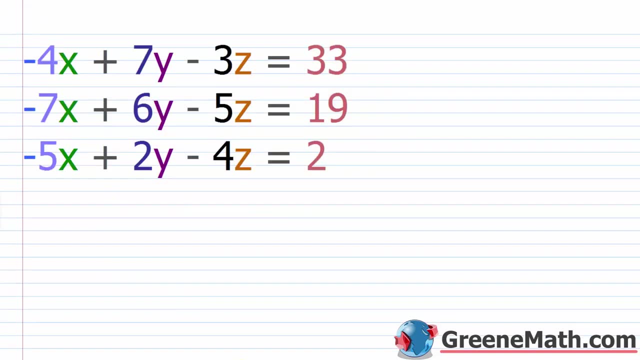 negative five. I can say that one Y equals three or Y equals three, And I can say that one X equals zero or X equals zero. All right, So let's continue with the next example. So now we have negative four: X plus seven, Y minus three, Z equals 33.. So negative four. 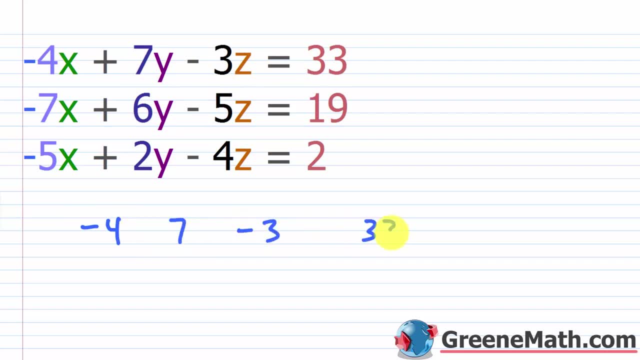 We have seven, We have negative three and we have 33.. Then we have negative seven: X plus six, Y minus five, Z equals 19.. So negative seven, six, negative five and then 19.. And then we have negative five: X plus two, Y minus four, Z equals two. So negative five, two negative four and two. Okay, So let 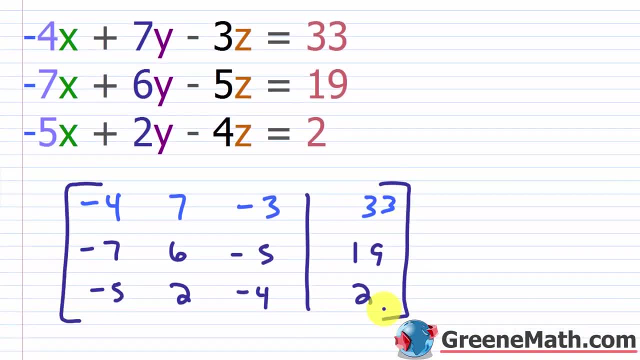 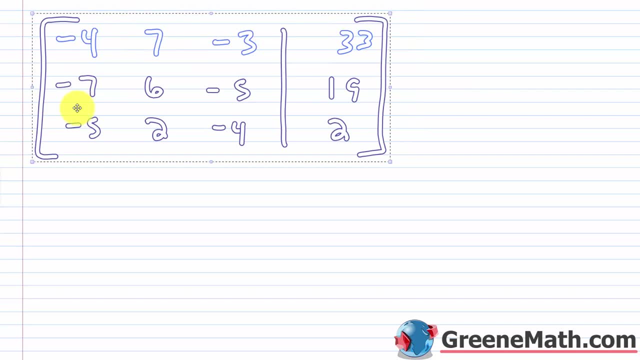 me put this bar here and then let me put these brackets and we're ready to go. So let me copy it to a nice fresh sheet. And again, we want one down the diagonal. We want zeros above and below. Okay, So I'm going to start by getting a one in this position here, And to do that I'm just going. 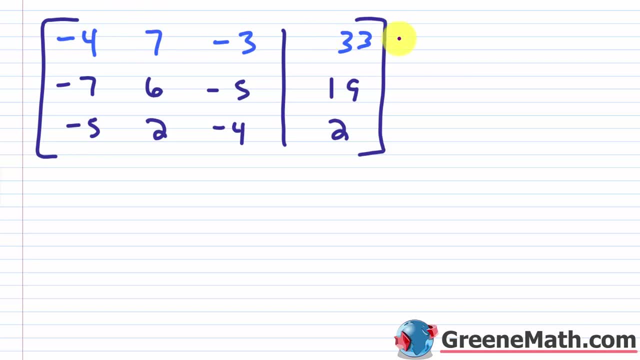 to multiply the top row or row one. Let me label these real quick, So row one, row two and row three. I'm just going to multiply row one by the reciprocal of negative four, So I'm going to do negative one fourth times row one. Okay, That's what I'm going to replace. row one: Okay. So now. 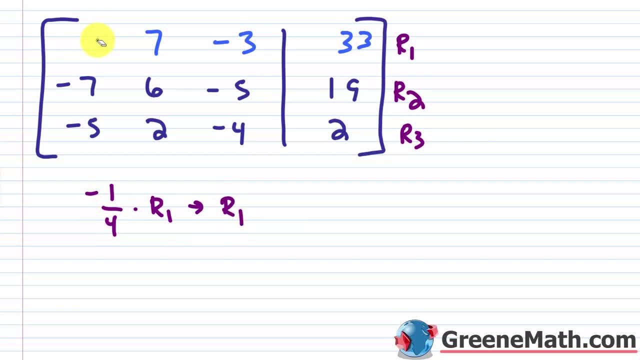 negative one fourth times. negative four is going to be one, Then negative one fourth times seven is going to be negative seven, fourths. So negative seven, fourths, Then negative one fourth times. negative three is going to be positive three fourths And then negative one fourth times. 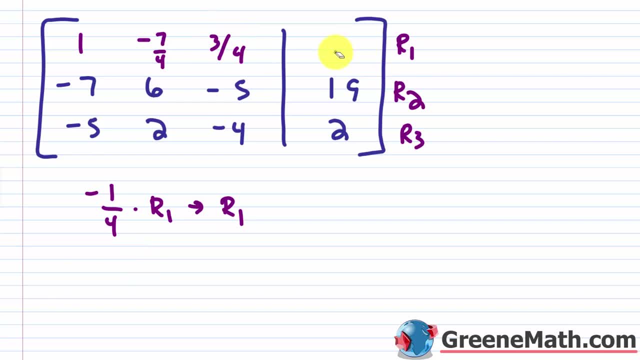 33 is going to be negative 33 fourths. So negative 33 fourths. Okay, So that part's done. So now I want to get a 0 here and here. So let me start with row 2 and getting a 0 here. So again, because 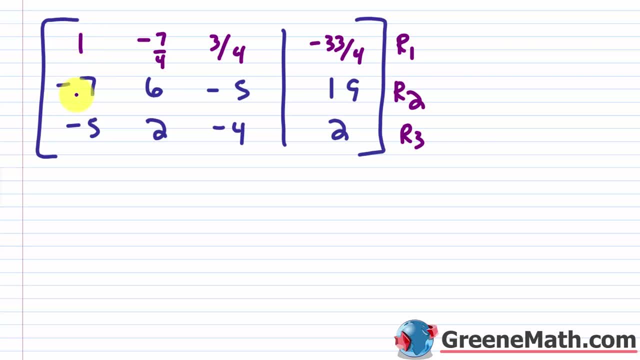 I have a 1 here. it makes it easy to get a 0 here, because I can just say: okay, I want to add a 7 to this negative 7 to get a 0. So I can multiply this top row or row 1 by 7.. So 7 times row 1, and then I 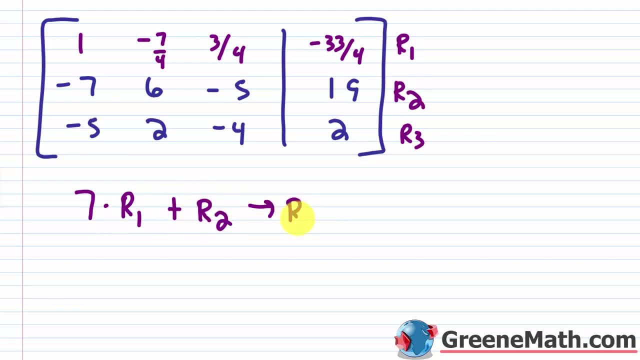 can add that result to row 2.. That's going to give me my new row 2, and this is going to be a 0.. Okay, so this would be 0.. And then, for this guy right here, I would have 7 times negative, 7 fourths. So 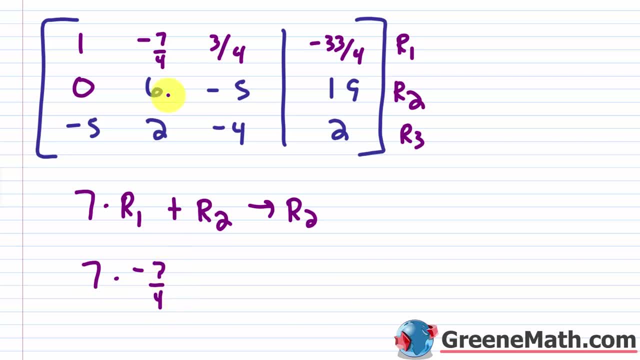 7 times negative 7 fourths, And then I would add that to 6.. So when that's done, I'm going to add that to 6.. So this would be negative 49 fourths, And then, if I add that to 6, I would make this 24. 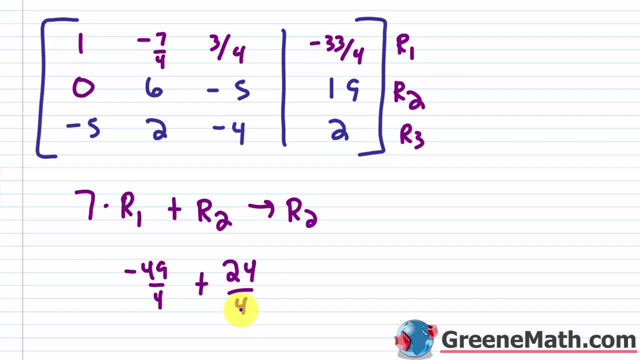 fourths. So this would end up giving me negative 25 fourths, So I'm going to put negative 25 fourths. Okay. so now I want to do 3 fourths times 7 and add the result to this negative 5.. 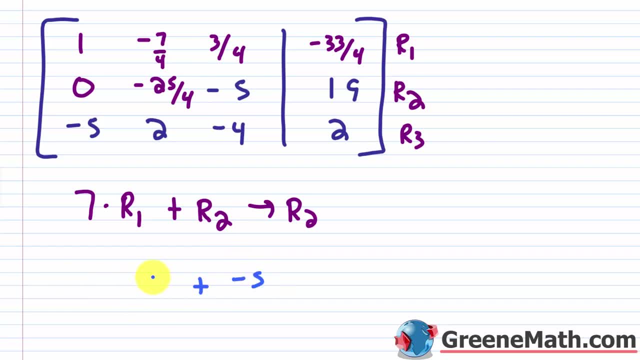 So this would end up being what It would be: 21 fourths. So 21 fourths plus negative 5.. So I can make this negative 20 over 4. And 21 plus negative 20 would be 1.. So this would be 1 fourth. Okay, so. 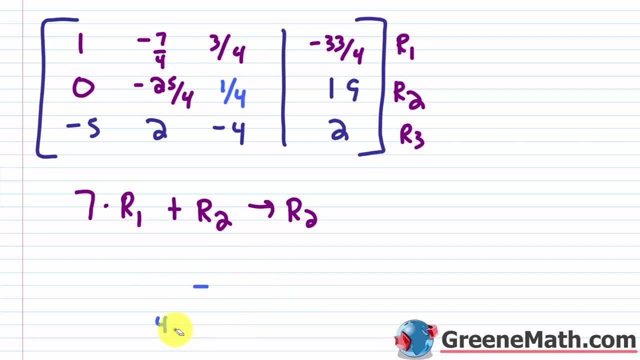 I'll erase this and put a 1 fourth here. So let's erase this. And then, lastly, I have this negative 33 fourths times 7. And then plus 19. when that's done, So this would end up giving me negative 231 fourths. So negative 231 fourths. 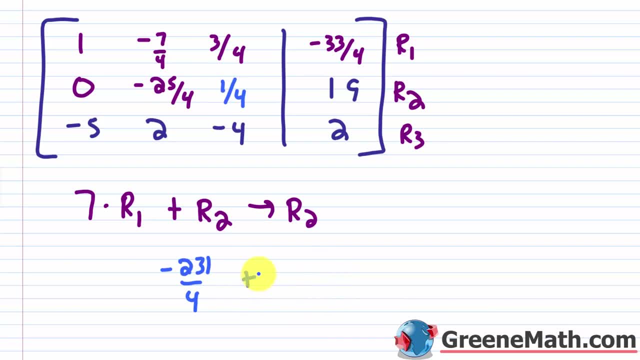 And then I'm adding to this 19.. Now what I can do to get a common denominator: 19 times 4 is 76. So I can say this is 76 fourths, So negative 231 plus 76. Is going to be negative 155. And this is over 4.. Okay, all right, so that part's done. Now we're. 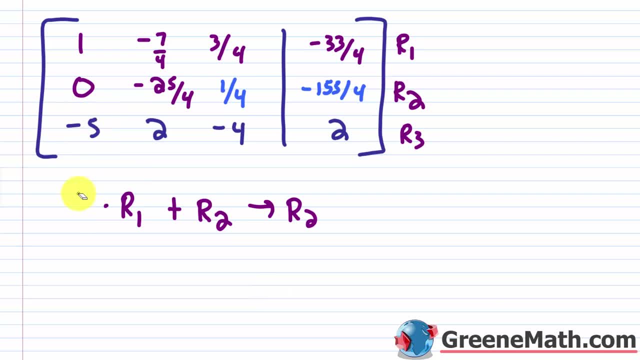 going to do something similar for this right here. So I would multiply 5 by row 1.. Again, think about that: 1.. 5 times 1 is 5.. Add that to negative 5, you get 0.. And I would add the result to row 3.. 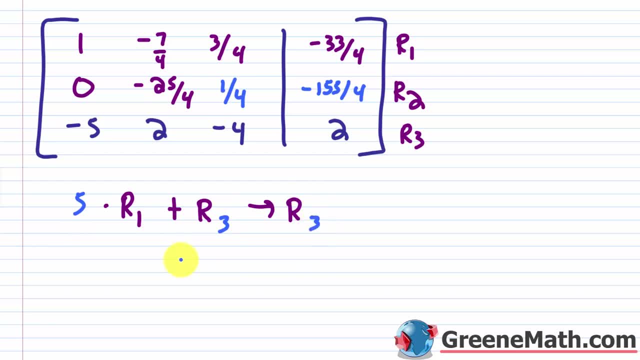 Okay, so that's going to give me my new row 3.. So if I do this, one would be 0.. So then I would take Negative 7 fourths And multiply it by 5. And add the result to 2.. So this is going to end up giving. 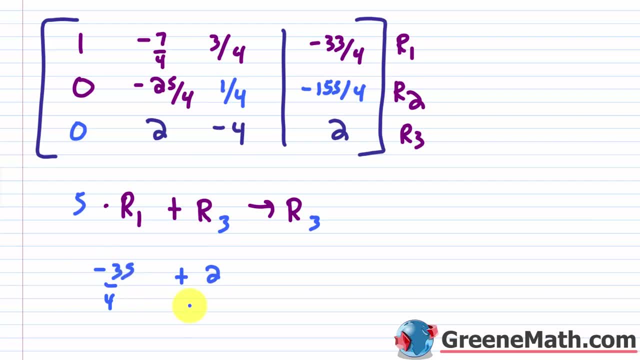 me negative 35 fourths And then plus instead of 2, I'm going to write 8 fourths. So negative 35 plus 8 is negative 27.. So this is going to be negative 27 fourths. That's going to go right here. So 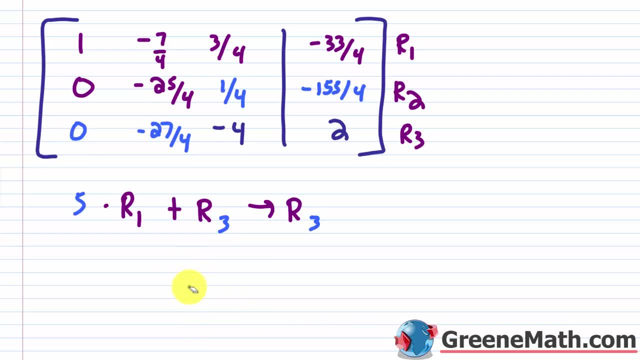 negative: 27 fourths. Okay, the next thing I want to do is take 3 fourths, So 3 fourths, and multiply it by 5. And then I'm going to add the result to 2. And this is going to end up giving me negative. 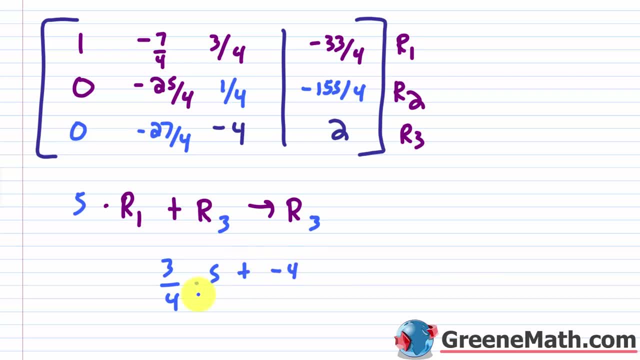 5 and then add the result to negative 4. so this is going to end up being 15 fourths. okay, and if i add this to negative 4, let's write this as negative 16 over 4. so 15 plus negative 16 is. 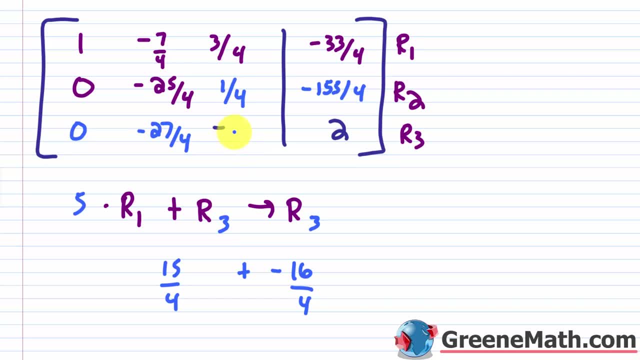 negative 1. so this will end up being negative: negative 1, 4th. okay, so negative 1: 4. and then, lastly, what i want to do is multiply 5 by negative 33 fourths. so negative 33 fourths times 5. 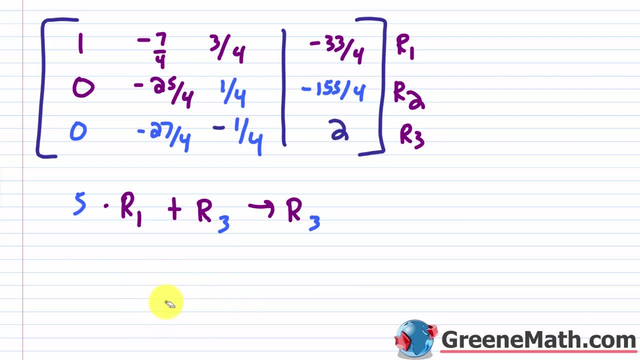 that's going to give me negative 165, so negative 165 over 4, and then plus 2 again. i'm going to write that as 8 over 4, so negative 165 plus 8 is negative 157. so this is negative 157 over 4 and 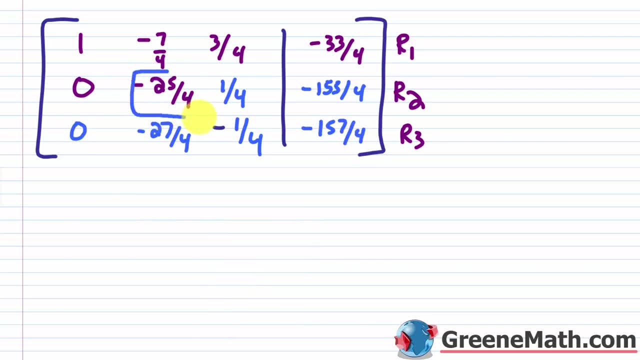 let's move on now. so the next thing i want to do is get a 1 here. okay, i always want to get a 1 first and then get my 0 below and above in this case, so i can do that by just multiplying row 2. 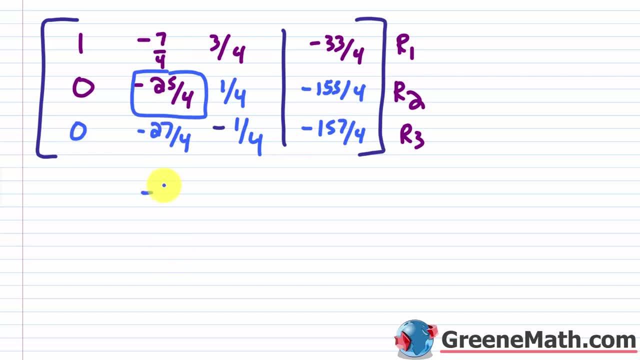 by the number of times i get a 1. so i'm going to do that by just multiplying row 2 by the number, the reciprocal of that, so I would have negative 4 25ths times my row 2. that's going to give me. 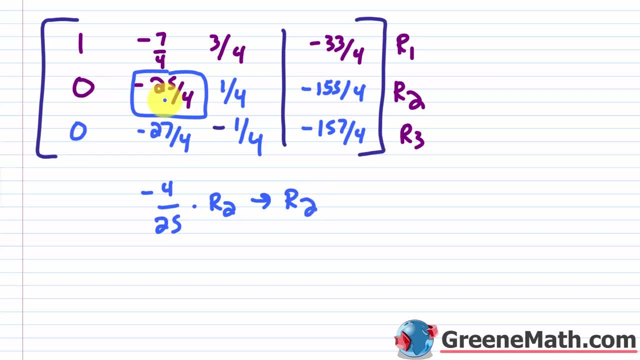 my new row 2: okay, so this is not going to be affected. this will turn into a 1. okay, this will be a 1. and then this guy right here: you'd have 1 4th times, negative 4 25ths. so what's going to? 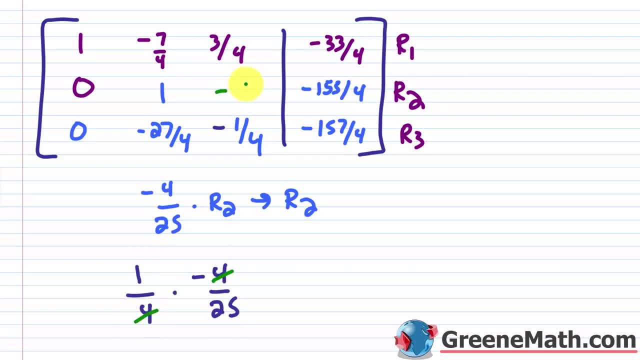 happen is this will cancel. with this, I'll have a negative 1 over 25. okay, and then let me erase this. the last thing I want to do is I want to take negative 4 over 25 and multiply it by negative 155 over 4, so this is going to cancel and you basically have this: negative times- negative. 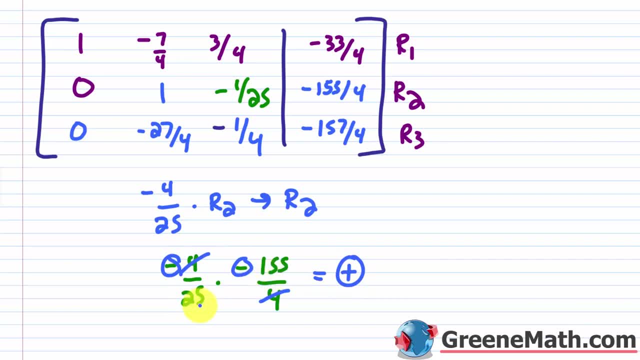 which would give you a positive between 155 and 25. you have a common factor of 5, so this would be 5 here and this would be 31 here. okay, so this right here is going to be 31 fifths, so let's erase. 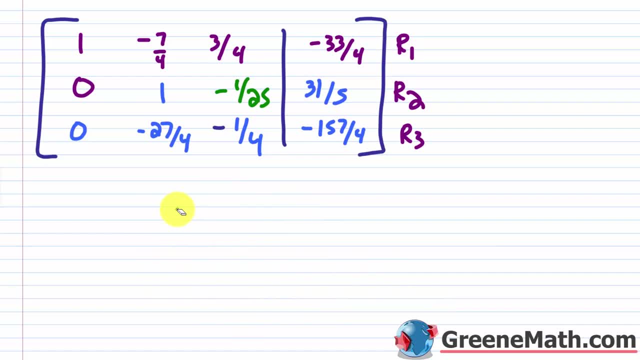 this, and then I'm going to take negative 4 over 25 and multiply it by negative 155 over 4. so this. so now we're done with that, and now I want to zero here and here. so to get a zero here on the bottom, I would multiply row 2 by 27 fourths. okay, so 27 fourths times row 2 and then plus row 3. 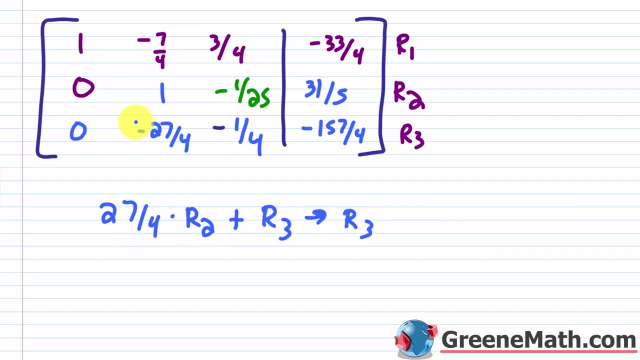 that's going to give me my new row 3, so again, I don't need to worry about this stuff over here. for this one. I know this is going to end up being a zero, so I'm really going to only have to work with kind of this part right here and this part right here, so I would have 27 fourths times. 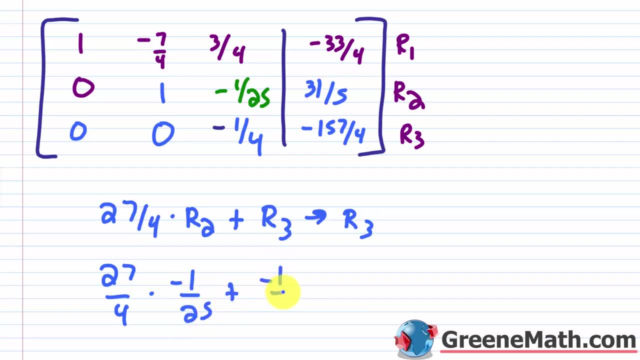 negative 1 over 25. so I'm going to have 27 fourths times, negative 1 over 25. so I'm going to have 27 over 25. I'm going to add that to negative 1- 4th. so what's going to happen is between 27 and 25. 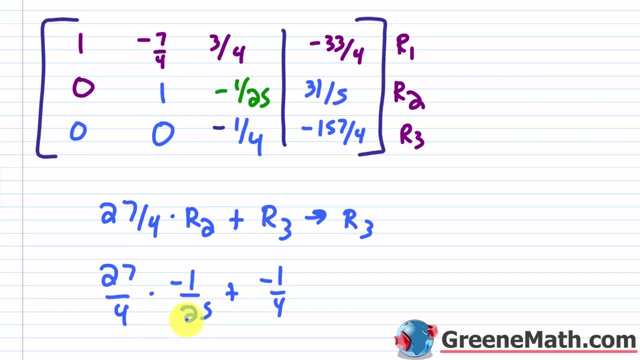 there's no common factors other than 1, so really I'm just going to say this is negative 27 over 100, so negative 27 over 100. for this I could multiply by 25 over 25, so I'd have negative 25 over 100. 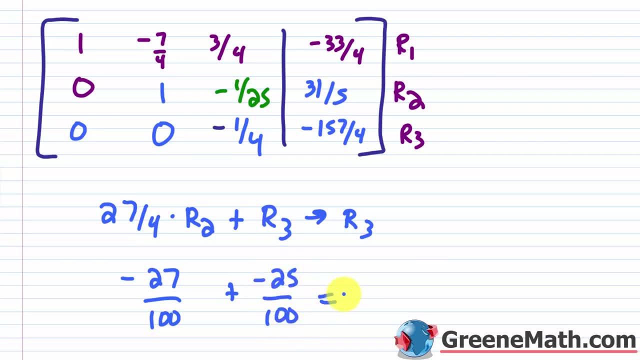 and that's going to give me what this would be: negative: 52 over 100. okay, so let me erase this and we can simplify this before we write it: 52 divided by 4 is 13 and 100 divided by 4 is 25. okay, so I'm going to write this as negative. 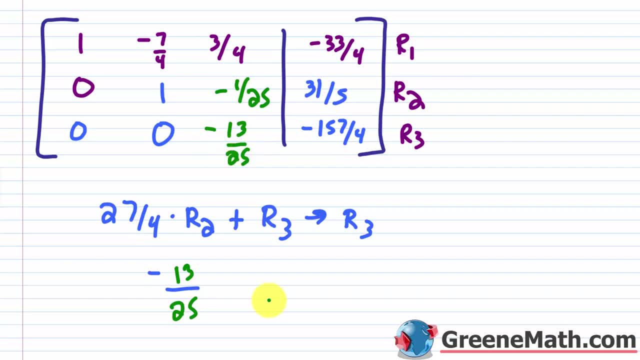 13 25ths, and then, lastly, I want to do 27 fourths times 31 fifths, and then add that to negative 1, 157 fourths. so 27 times 31 is 837. so this would be 837 over 20, so 837 over 20 if I multiply this. 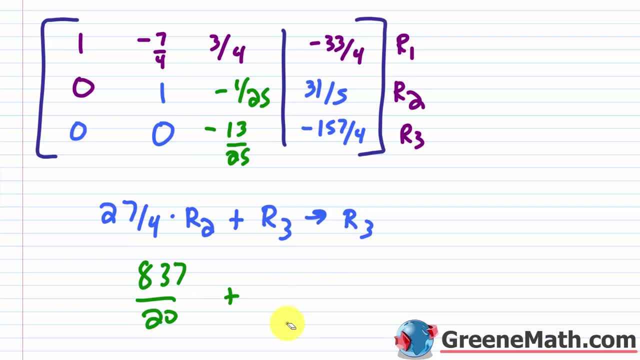 by 5 over 5, I would get negative 785 over 20. so if I do this, addition 837 plus negative 785, I'm going to get 52. okay, so I would get 52 over 20, 52 over 20, which is going to simplify each is. 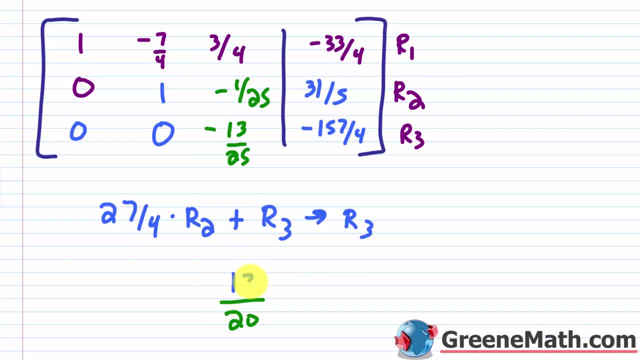 divisible by 5, so I'm going to get 52 over 20. so I'm going to get 52 over 20, which is going to be divisible by 4. 52 divided by 4 again it's 13. 20 divided by 4 is 5. so this guy right here is going. 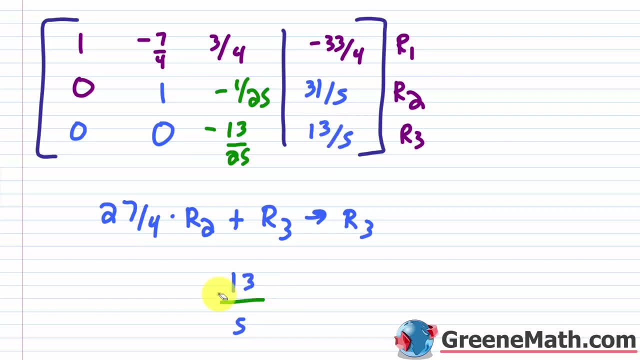 to be 13 fifths. okay, all right, so let's work on this and getting a 0 here. so again, I want to multiply row 2 by 7- fourths now- and add the result to row 1. okay, that's going to be my new row 1, and 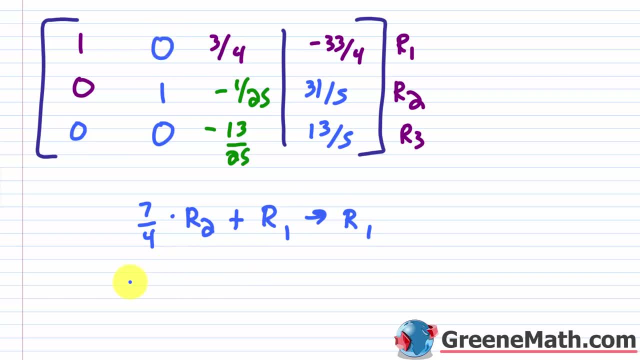 so I already know that this is going to be a 0. okay, then you would have 7 fourths times negative, 1 over 25. add that to 3 and that's going to be my new row 1, and so I already know that this is. 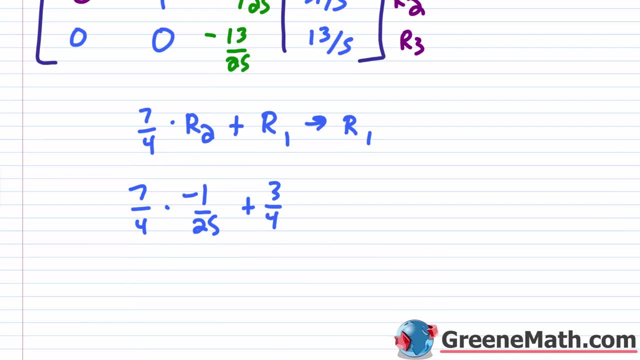 going to have a 3 quarter decimal again. so we're going to add the result to row 1 now and I'm going to have to. let's goodness me, what is this going to be5. this here, first one, I told myself would be 3.15, let me scroll down a little bit. I'll come back up. let's quote this right here- would be: 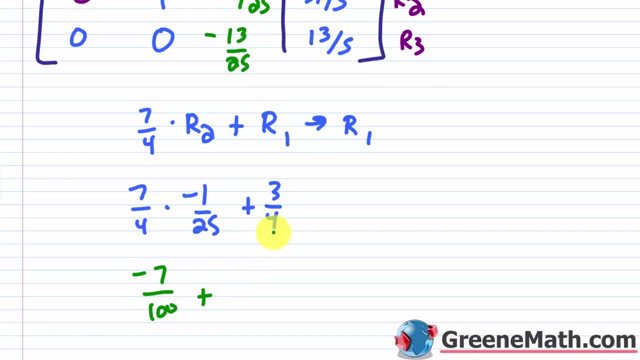 negative 7 over 100 plus. if I multiply this by 25 over 25, I would have 75 over a hundred. negative 7 plus 75 is going to be 68. so this would be 68 over 100 plus if I multiply this by 25 over 25. I 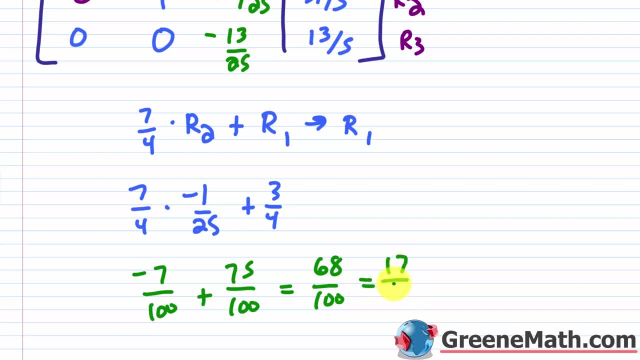 would have 75 over a hundred. negative 7 plus 75 is going to be 68, so this would be 68 over a hundred, which would simplify: 68 divided by 4 is 17, so this would be 17 over 25, right, because 100 divided by 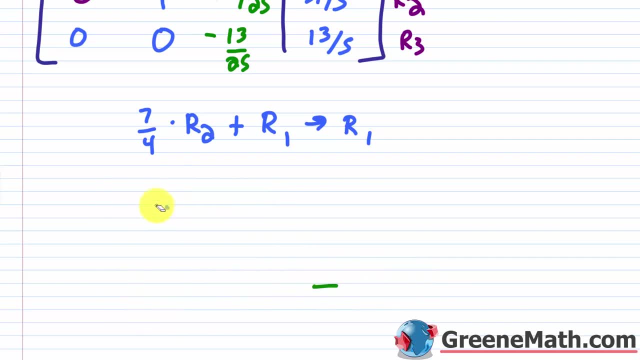 4 is 25, so this would be 17 over 25.. so I'm just going to add the more, which is I'm just going toancyears, so 17 over 25, and then for this one right here again, we're going to multiply 7 fourths times. 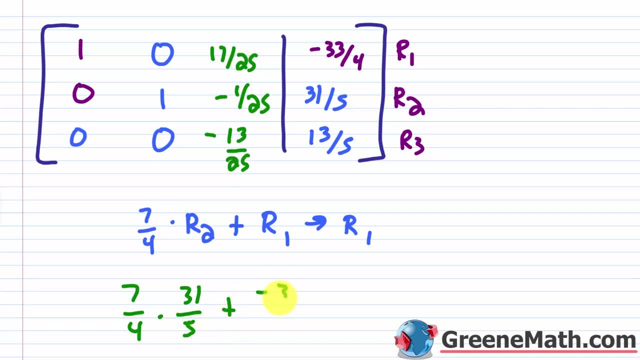 31 fifths, and then plus negative 33 fourths. okay, so 7 times 31 is 217. so you'd have 217 over 20, so 217 over 20, and i'll multiply this by 5 over 5, so this would be negative 165 over 20. 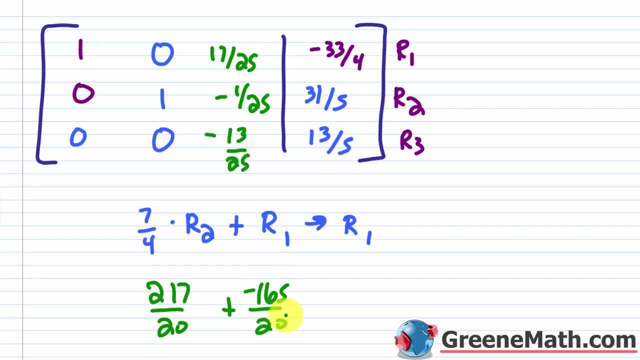 so 217 minus 165 is going to give me 52, so i'd end up with 52 over 20. so 52 over 20, and we already know this is going to simplify to 13 over 5, right, because 52 divided by 4 is 13 and 20. 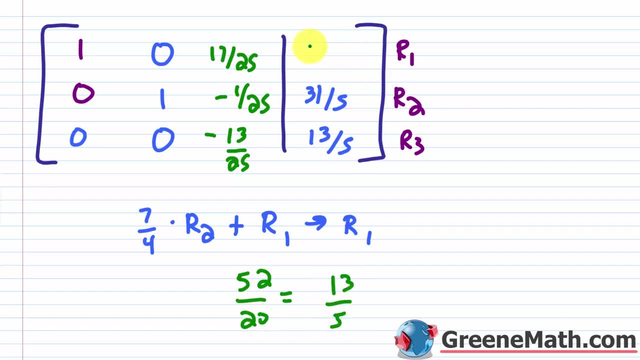 divided by 4 is 5, okay, so i'm going to replace this with 13 fifths. so now i want to move on to this column and i want to get a 1 here, okay. so how do i do that? i multiply row 3 by the. 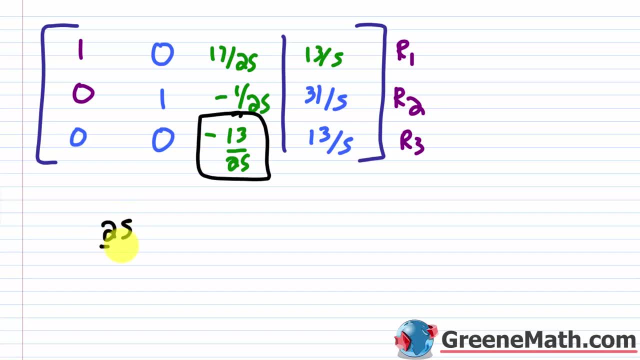 reciprocal of this. so i would take 25 over 13, the negative of that, multiply it by row 3. that's my new row 3. again, this one and this one are not going to be affected. this guy is going to be a 1, and then this guy right here. i'd have negative 25 over 13 times 13 over 5. the 13s are going to. 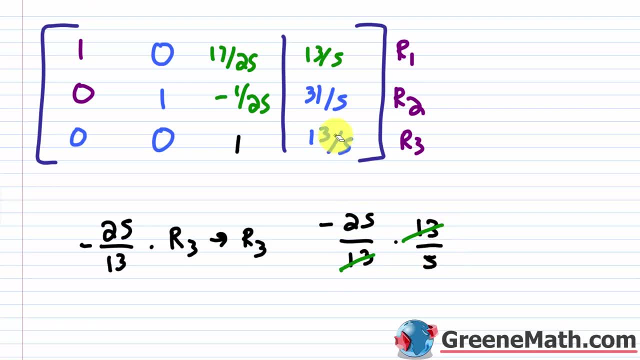 cancel. negative 25 over 5 is negative 5. so this is negative 5 and at this point again, you could go back and substitute. you know z is negative 5. at this point you could find out x and y. but we're going to continue, we're going to get a zero here and here, okay. so what i want to do to make this: 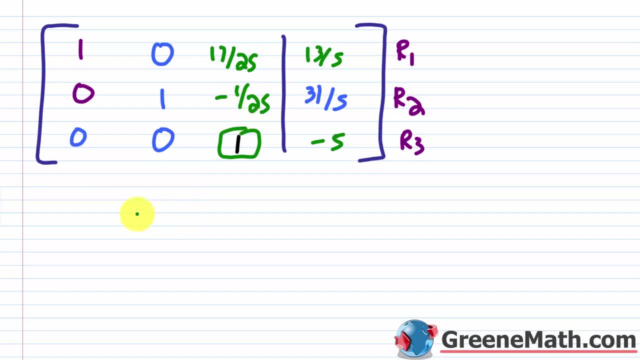 into a zero. i want to use this one here. the additive inverse would be 1 over 25, so times this row 3 and then plus row 2. okay, so i know that i don't need to worry about this or this, because multiplying by zero would leave a zero, and then adding zero to that would leave it.